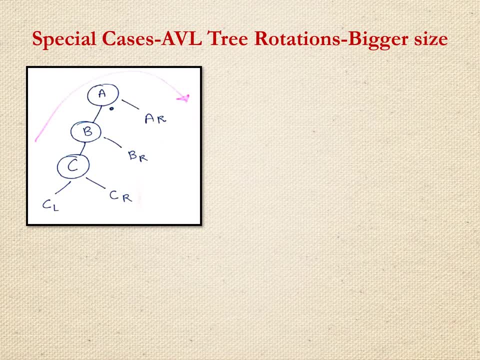 And CL. that is a left child of C And CR is a right child of C. So we can, if we'll be doing. if suppose your node A becomes here imbalanced, So it'll be. it's a left-left imbalance. So how we can sort it, We have to shift it A to the right and then B will become the root node and C will be on the same position. But let us have if we'll have some problem in this while doing the rotation. 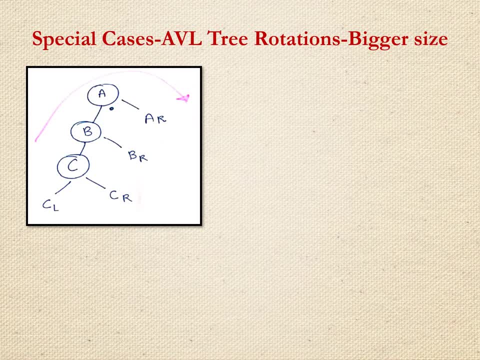 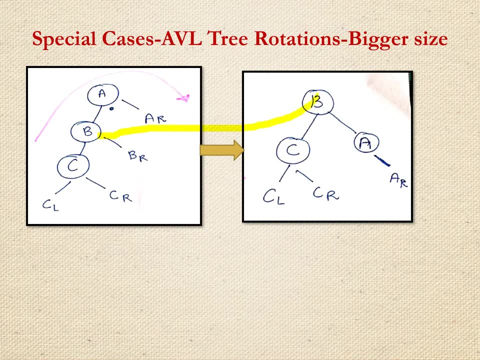 So we are doing the LL imbalance. So we'll be getting here: The B node will be there, that B will be then the root node and A shifted to right. So now A shifted to this right. So your A node is as it is and C is on the same position. Okay, So now let us understand that the CL and CR, these nodes are as it is here for the, as a child node, for C node. 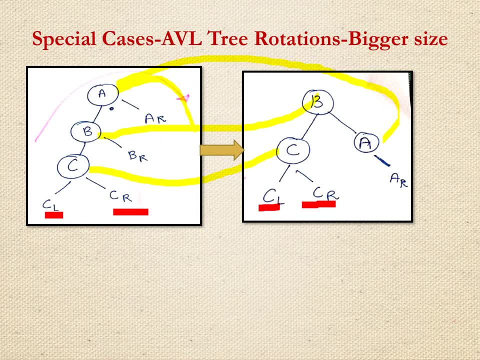 Then for a node, that is, we can say the a's, that a? r, that is the right child of your a node is also the same on the right hand side. now what will happen? but b is a root now. so how will be putting this b? r, this right child of the b node, where, where we can put it? so you can verify the difficulty. 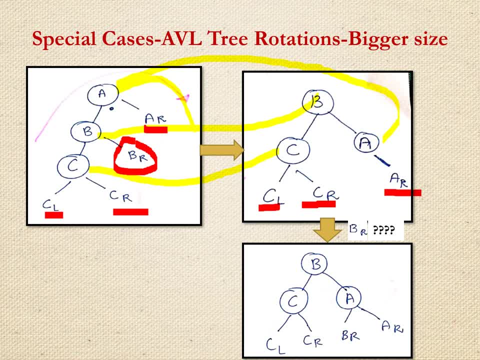 that is placement of b r. so your b? r will be shifted as the left child of your a. so now this b? r is shifted here as a left child of a because this b? r was right to your, that root of your, that a and that way their position that is identified. it is, that is a. 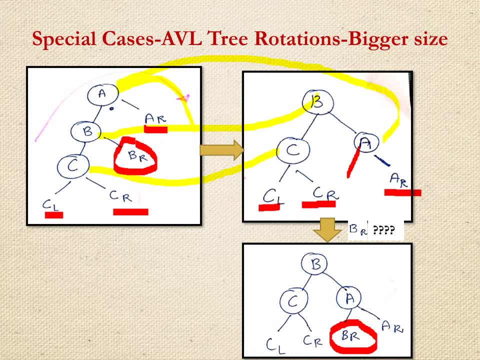 left child of your a. so we can say that this is just a small, what we can call it as a special case when we when we'll do some kind of rotation as for a bigger size. so this was again a left left imbalance, because we have started from this point. it was a left imbalance. again here it is a left imbalance. we have already. 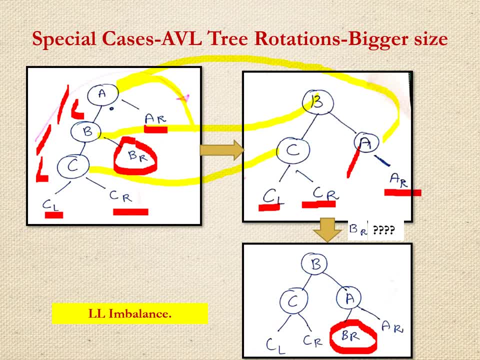 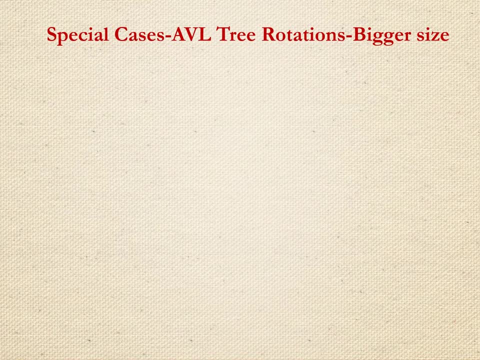 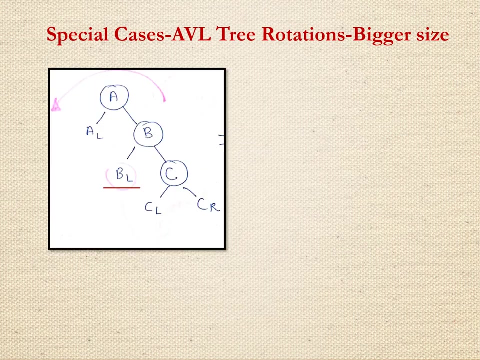 seen this ll as a rotation in the previous video. for better understanding, you can refer that video also. so proceeding further now, now again, it's an imbalance again, the same kind of what you can call it. at the children's are there for every node: al is the left child of a, bl is the left child of b, and cl and cr are the both. 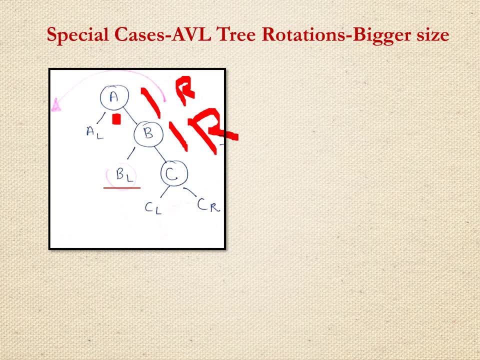 childs of c node. now we'll be shifting. this is rr imbalance, so we'll be going left side. so what will happen in this case? b will be, b will become the root node, a will be shifted totally downward here and c will be as it is now. what will happen with the left child of a is the left child of b. 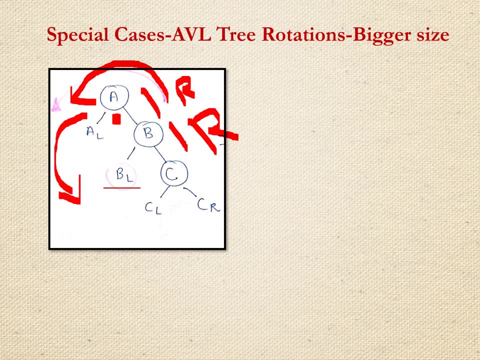 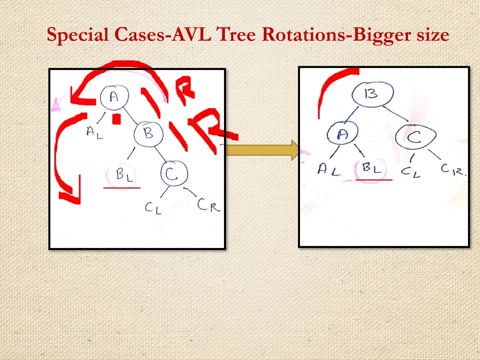 is the left child of plugc node and this is the first time we can go forward discussion tier 3 and c. this in this case is a left child of a. so now these are the left kinds of nodes. they're allels also. we can call them similarly and the same time we are, nodes should also be. 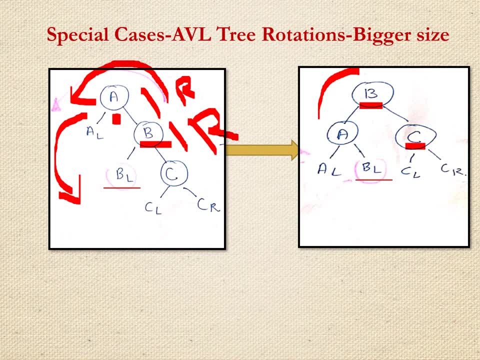 named themes of left node c and also how it's working. we are using them. we're going to call al requests n als a child of c, which means if you want, you can write it as the child of a, and if you all want to open all, let us verify that you can put a child of c or yet. you can put another child of c, or else? do you know that? what would that be? and now again, we are placing a child of a and E for these nodes alone. so so this is the function of the rightlle side, and then this is the left child of nodes, and then c is there as 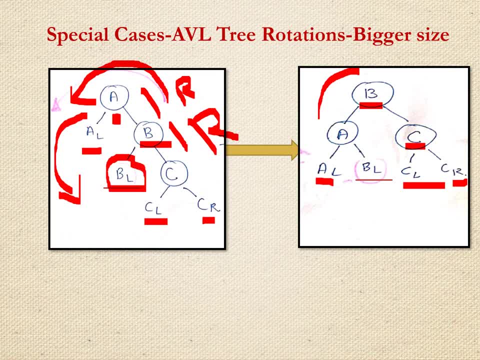 as it is. what about, then, this B? so B plays here the important role where the B will be shifted. so again, B will be shifted to the right child of your that A node. why? because this BL was right to towards B and then this position, so again A is now. this BL is shifted to the right of your B. 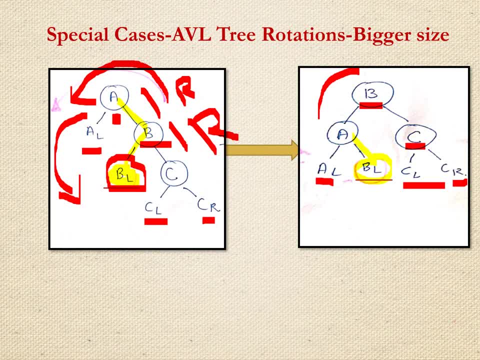 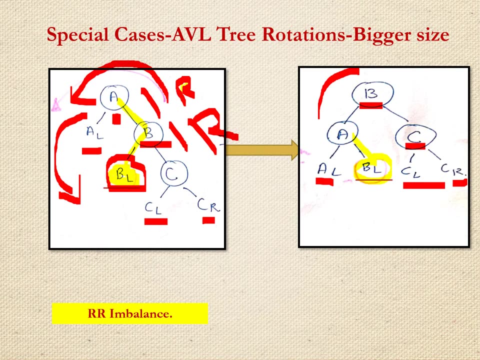 so you can verify that BL is placed here. so this way we can find some of the special cases while understanding the rotation in avial tree. let us go ahead. so the again. this was a right right imbalance. already I have explained it. it is a right right. 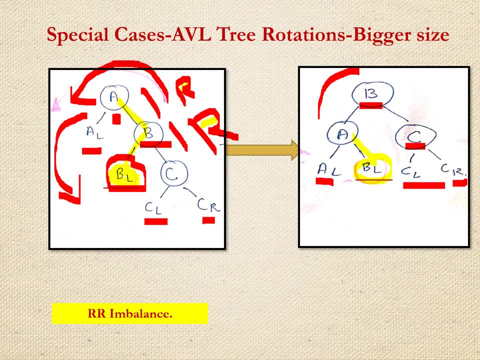 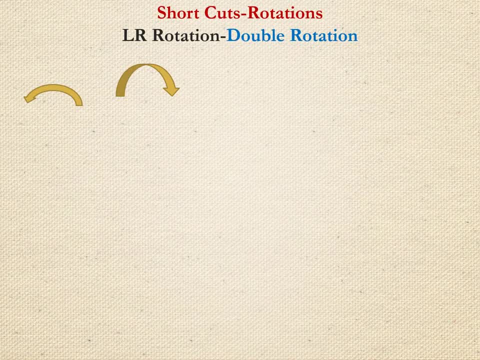 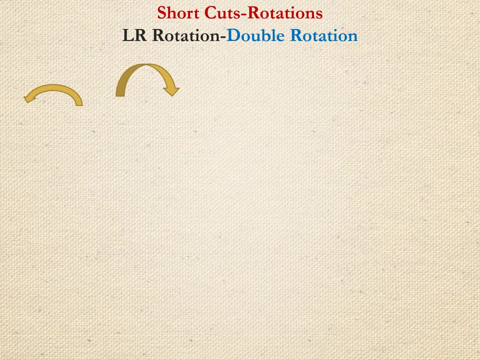 imbalance because it was because of this right node, that is, C was right to the B and B was right to the A. now let us understand some more. you can verify that BL is placed here. so this way we can find some of the special cases while rotations, or we can call it as the lr rotation or double rotation. but some shortcuts will be. 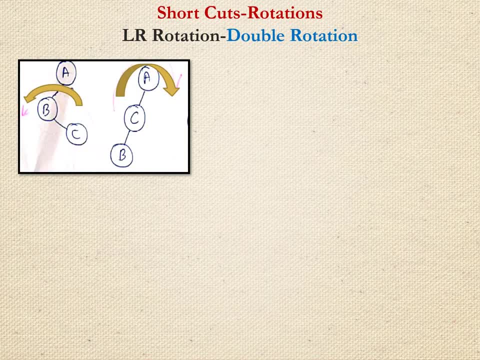 using it. so now suppose we were having this kind of what we can call it as the lr rotation. so what we do it? we first do the left l, that is, on the left hand side we rotate the node, and then on the right hand side we rotate the node, in this case for the three nodes abc. 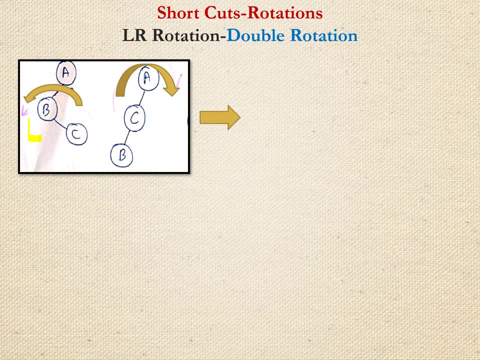 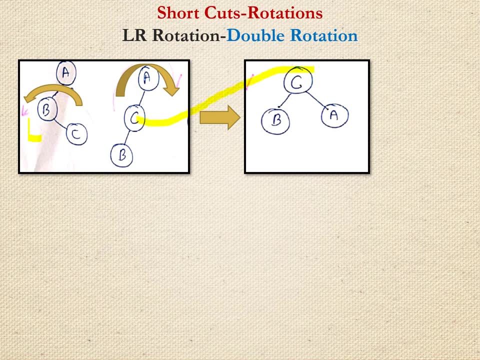 so the resultant what we get out of it is that this one means we will be getting a total shifting, that c will become then a root node and then b is the left of your this c and a is the right node of your c. so now, this way we get the arrangement. so that means when 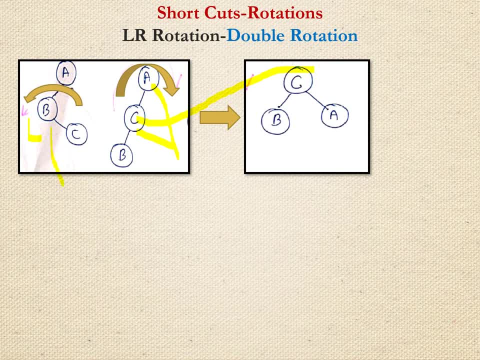 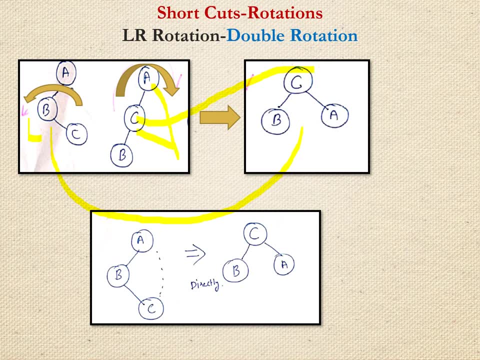 we do have this kind of lr imbalance so we should have this arrangement directly so we can find a shortcut directly that if we do have this kind of arrangement, that means we can do this- we can replace this c node directly to your root node and then you can place c. 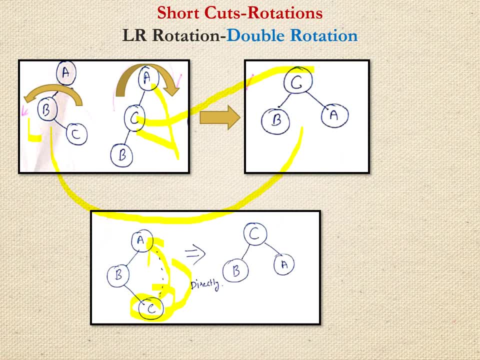 on the right of it. okay, that means c will be replaced there and a will be then on the right of way. so this is that way. so you replace c with a. b's position is as it is. only c is replaced at the root position and this a, this a, will be shifting towards the right, okay. 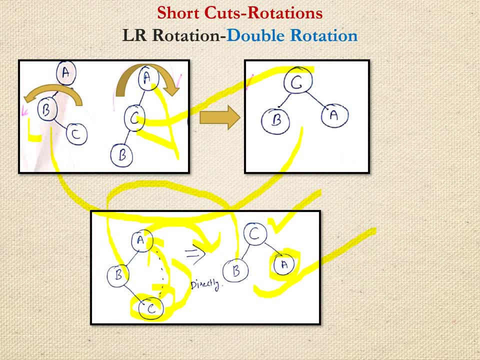 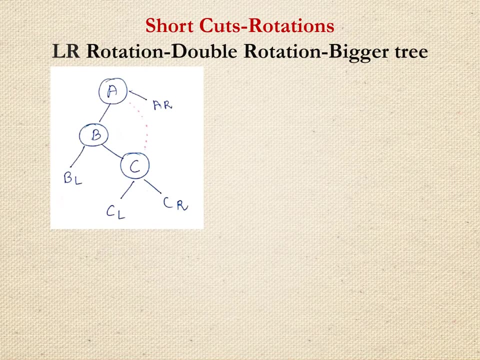 so this way we can do, or we can find some of the shortcuts for the double rotations. similarly you can find the shortcut rotation for the RL rotation also. so now, here again it's a again shortcut for the bigger tree. we can verify for the LR rotation. so suppose, if this is a case, that this is left and right and we 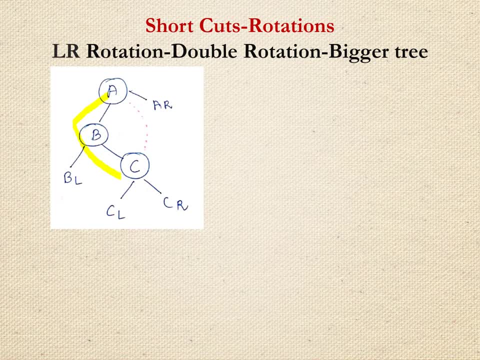 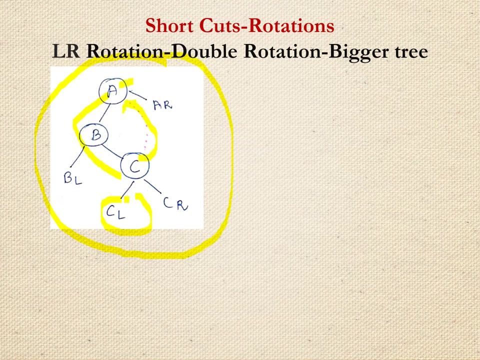 have to do it. and now the same LR rotation. it is now for the bigger size. now the tree is little bit bigger because it's having the different child's with it. so now, if this is the case, then what we can do again, C will be taking the position of your a node and a will be on the. I mean C will be here and 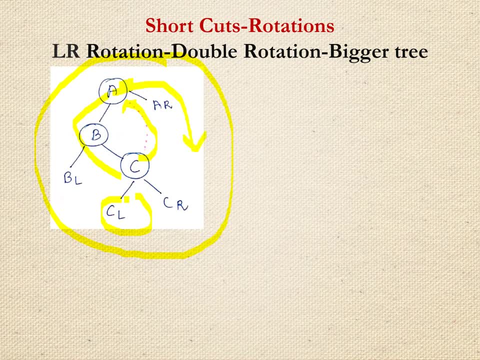 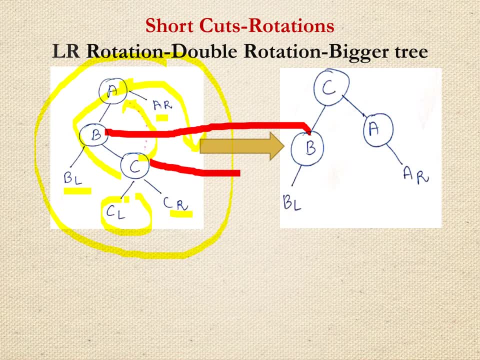 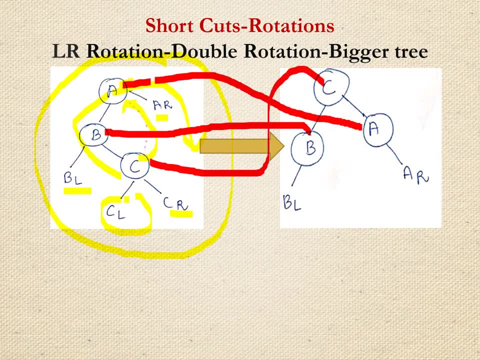 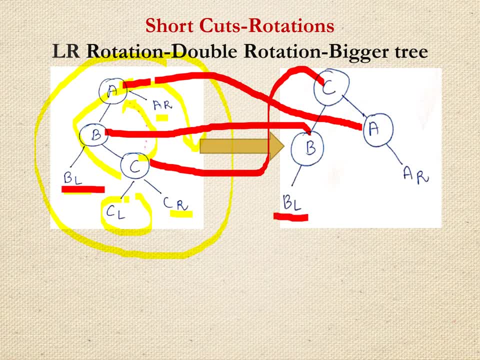 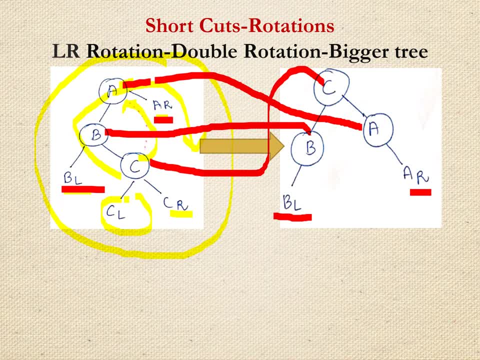 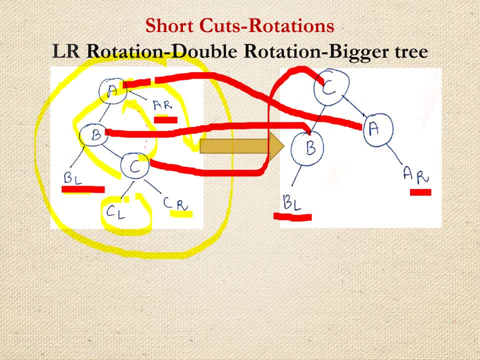 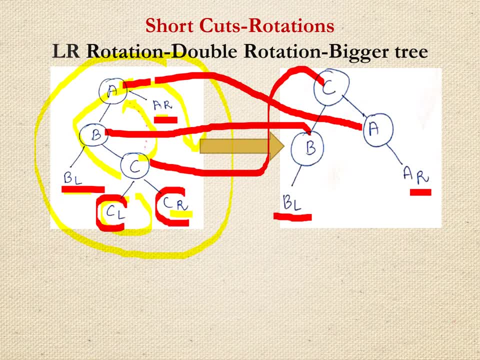 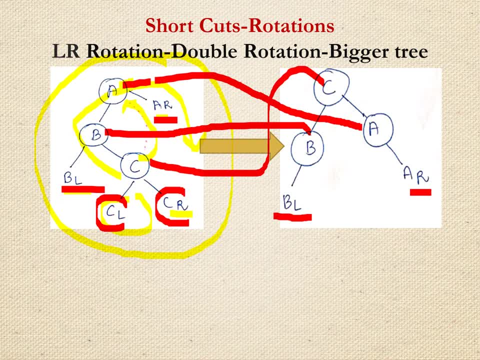 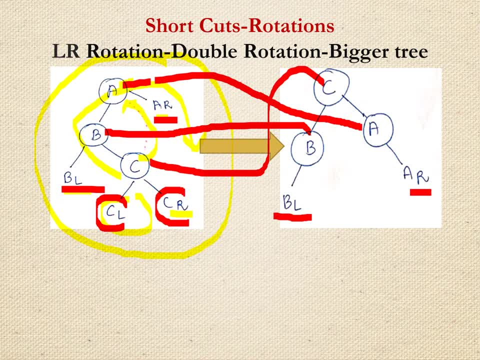 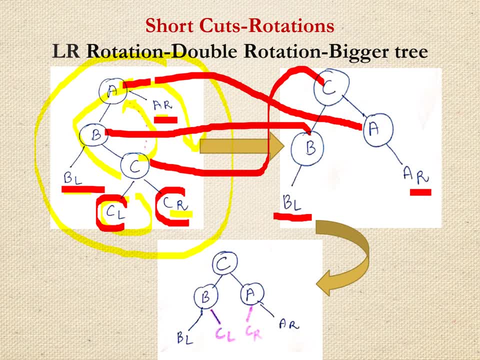 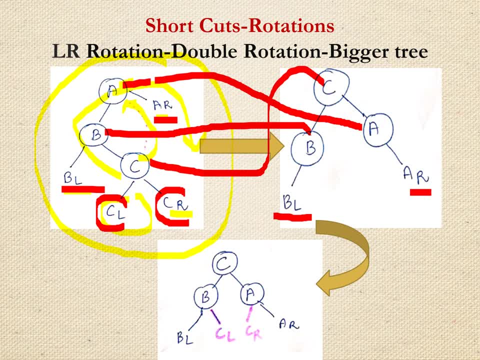 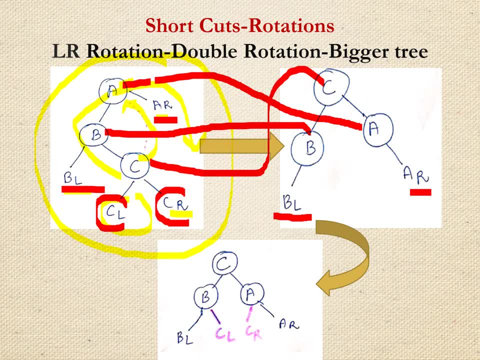 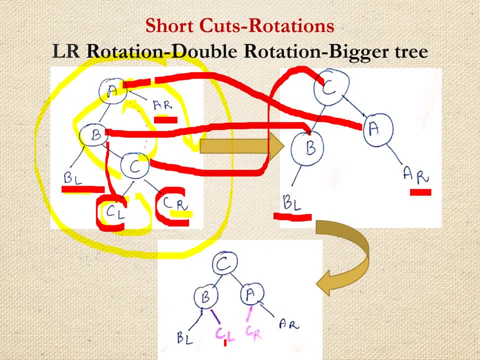 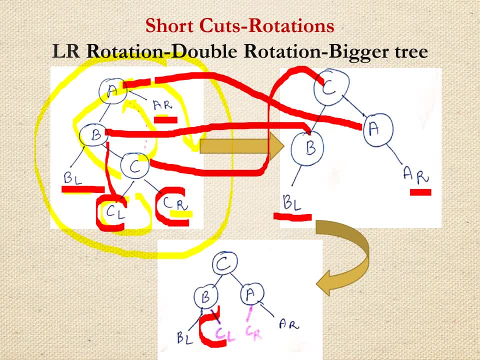 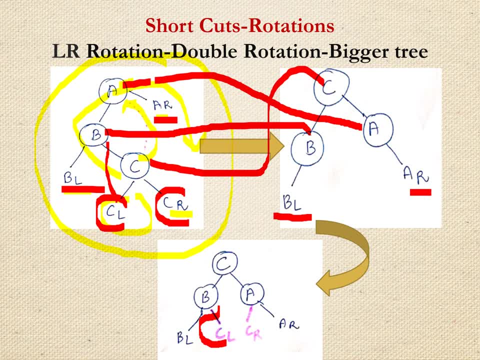 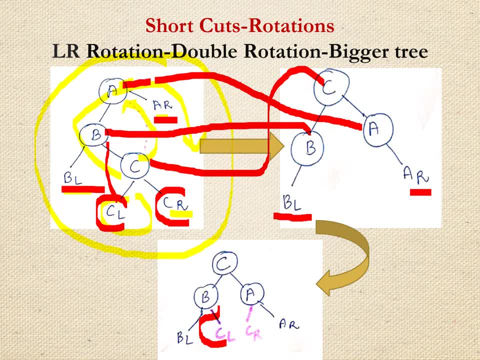 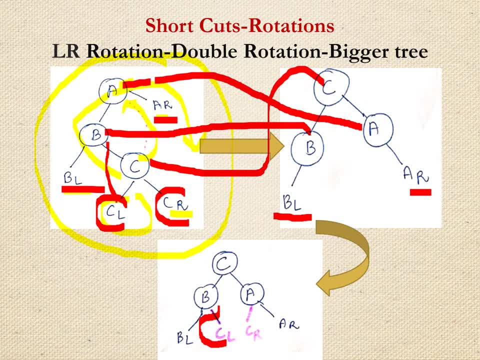 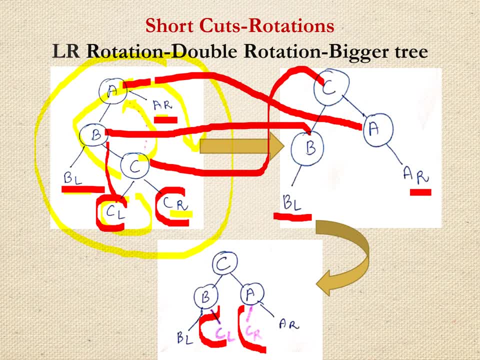 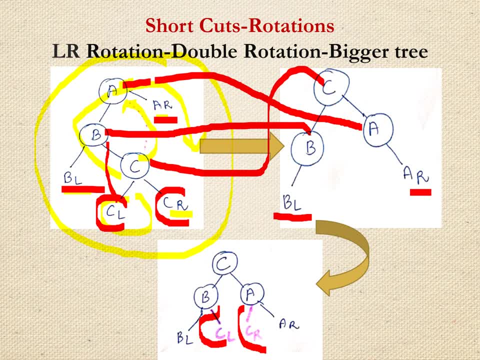 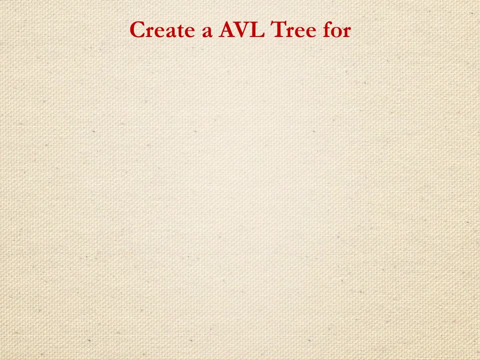 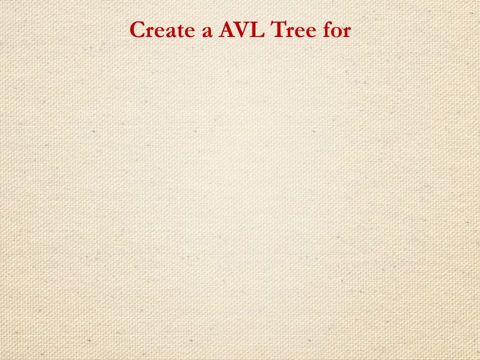 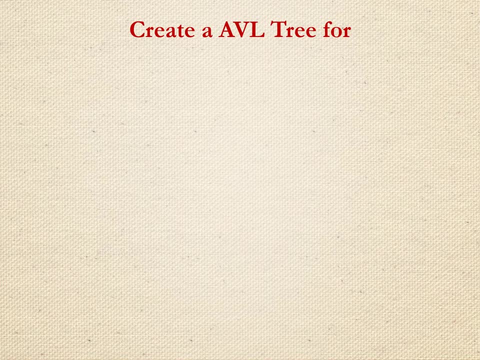 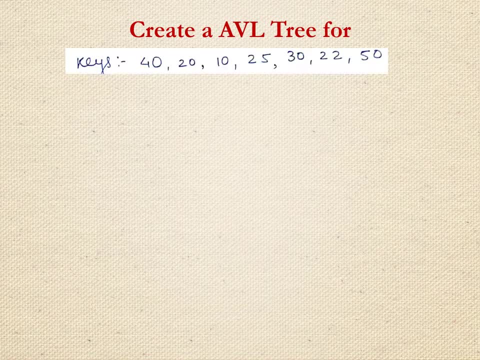 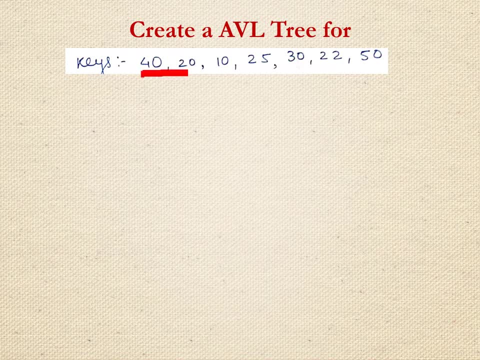 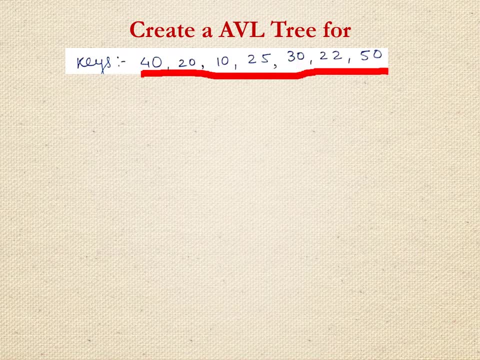 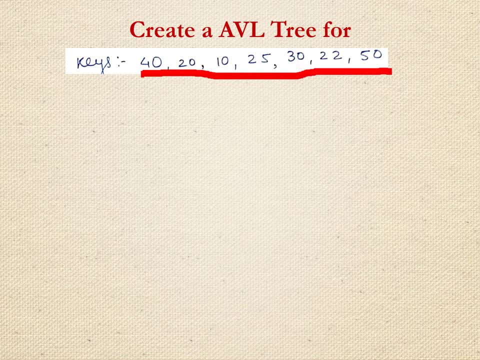 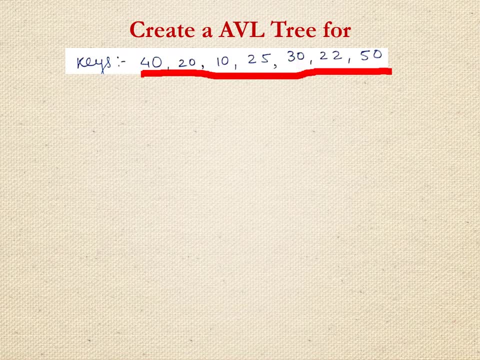 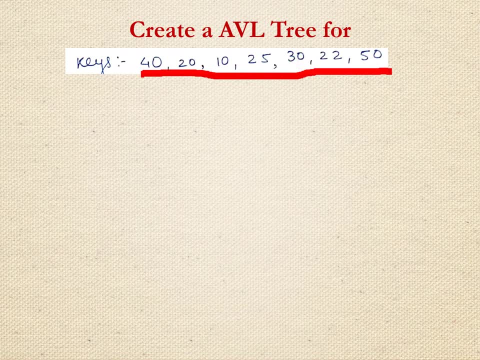 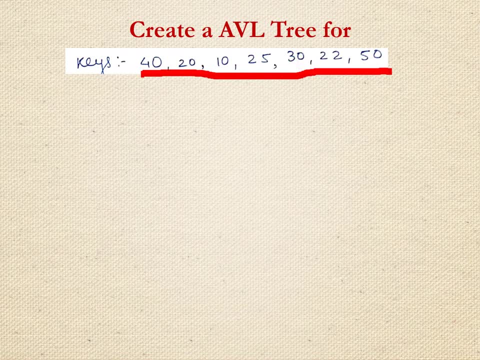 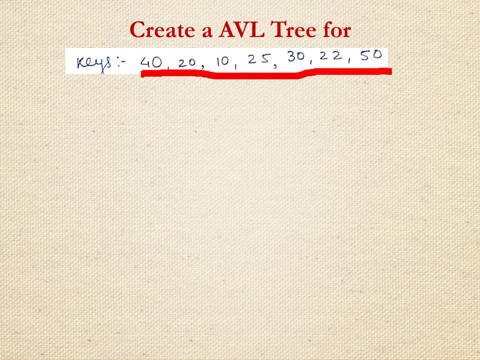 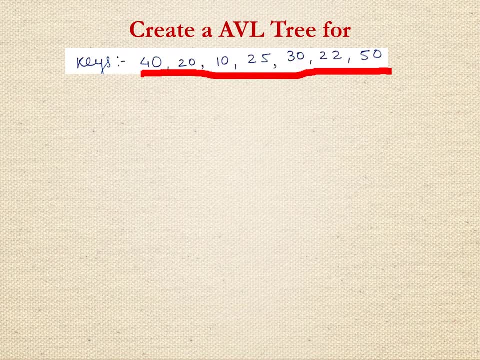 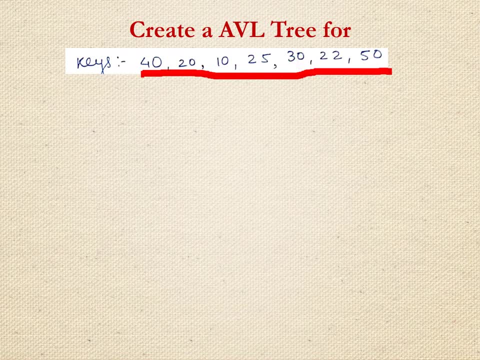 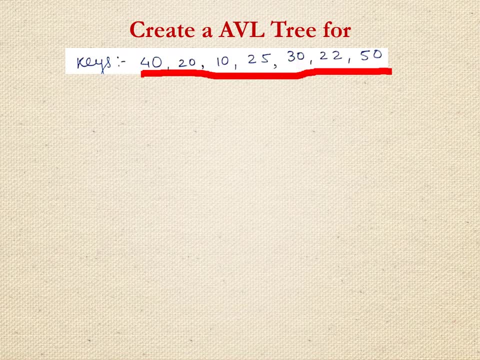 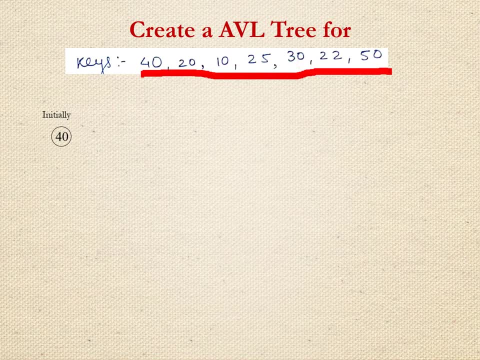 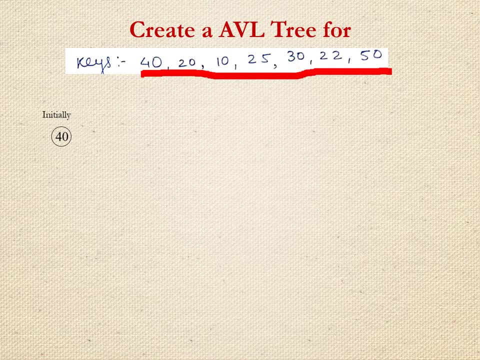 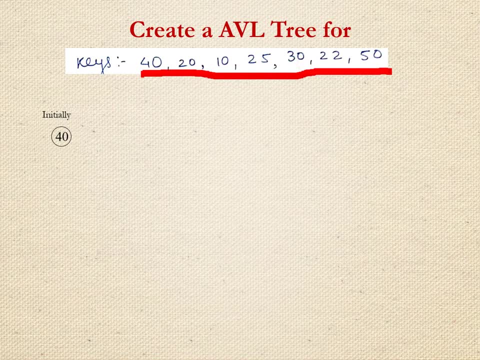 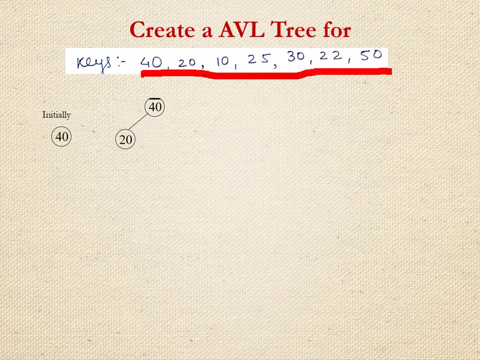 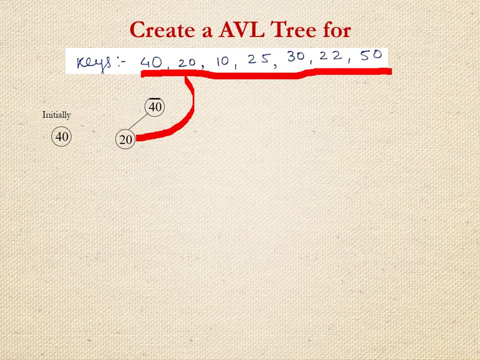 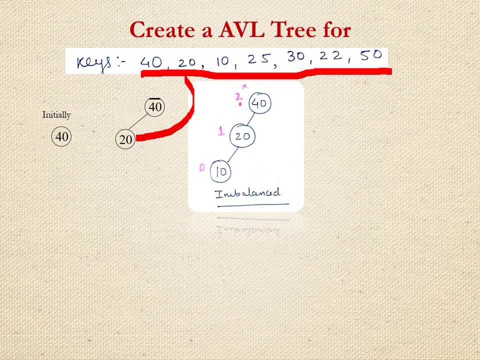 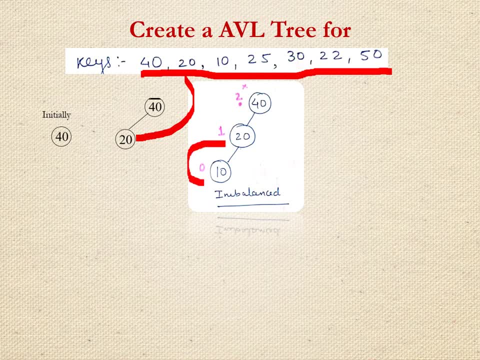 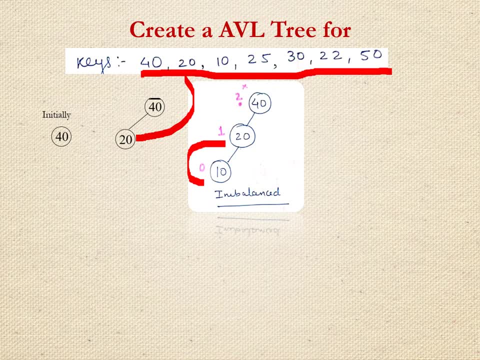 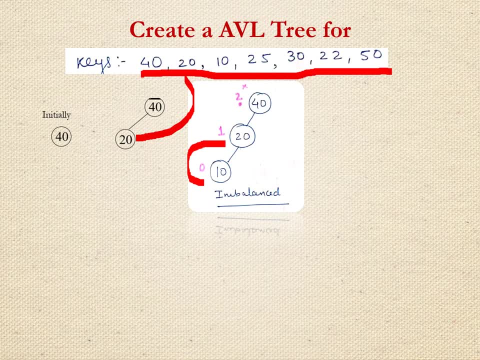 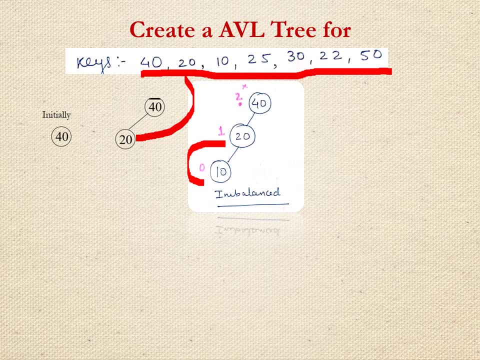 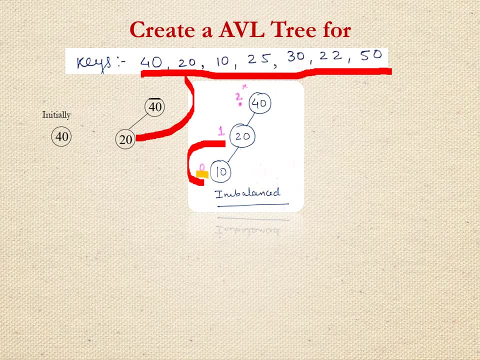 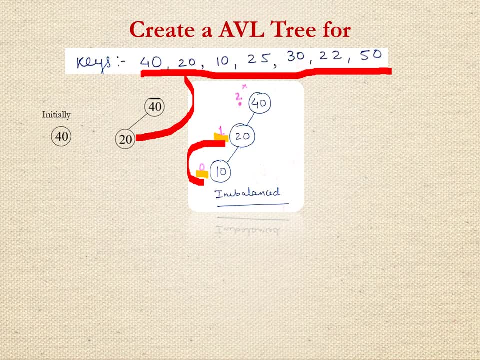 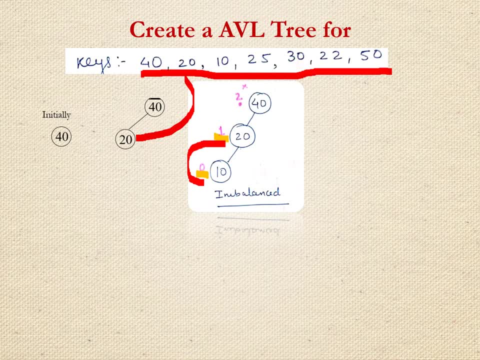 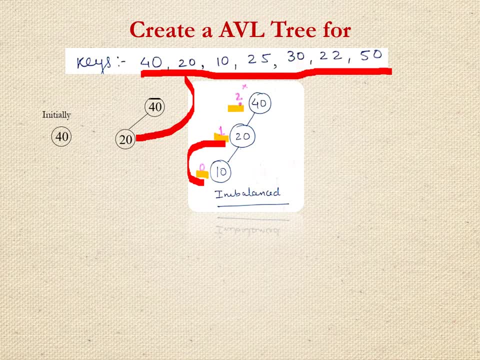 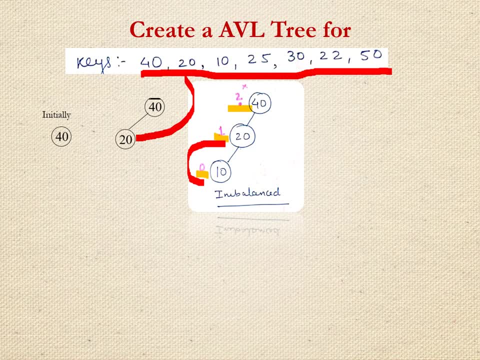 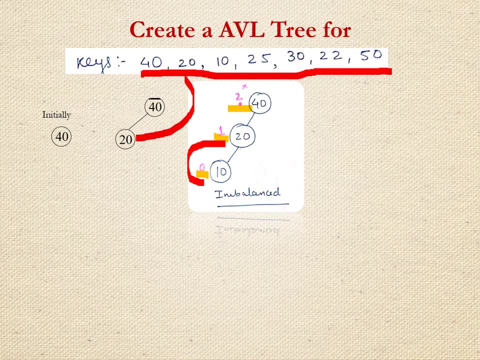 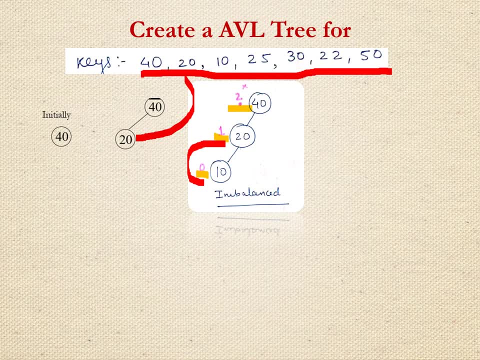 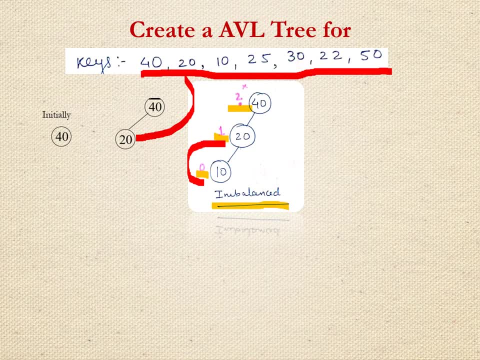 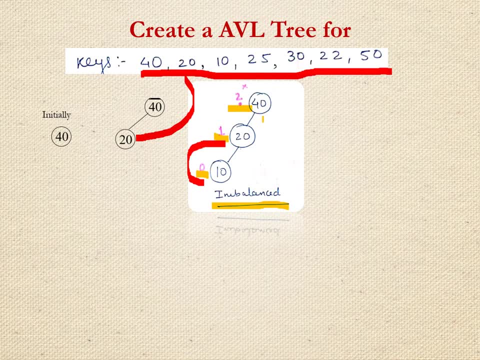 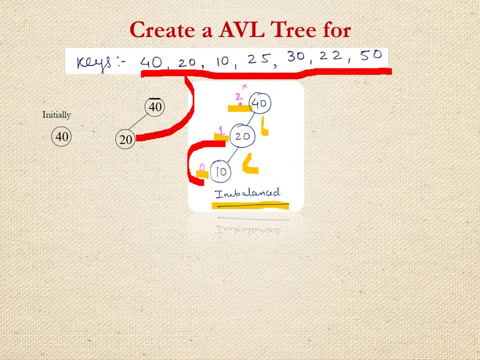 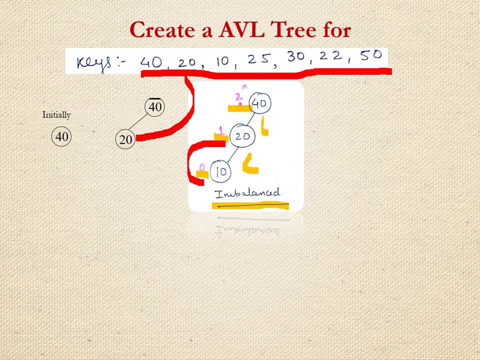 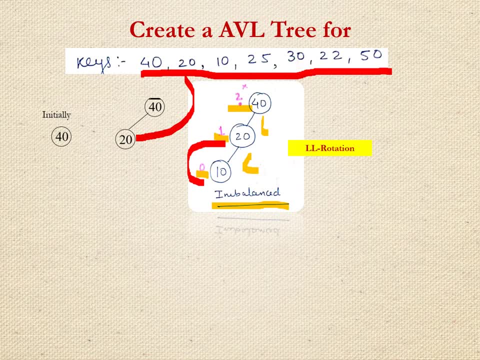 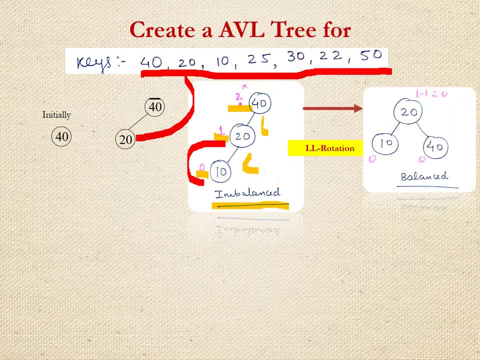 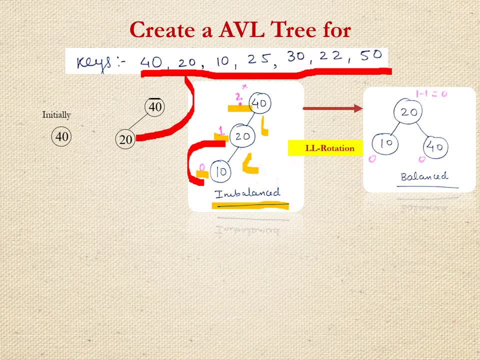 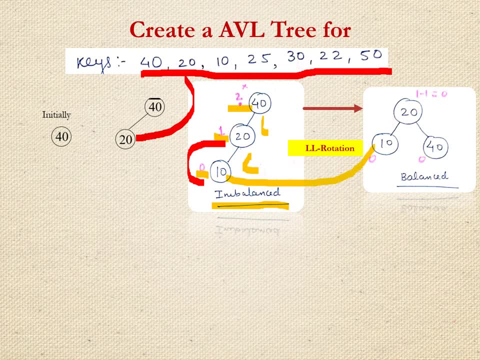 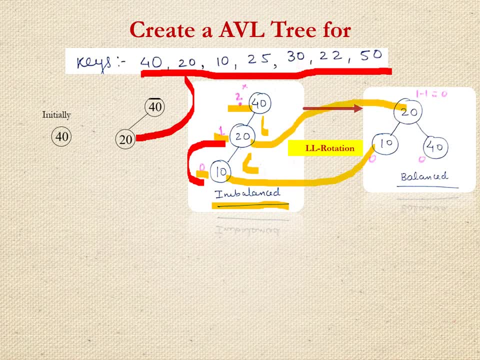 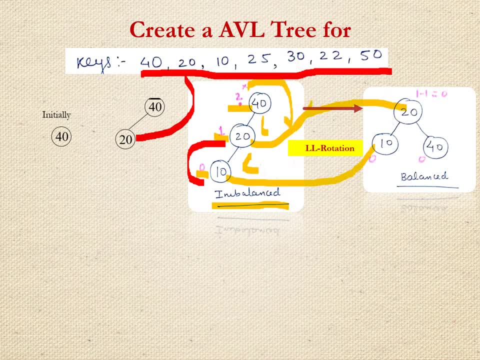 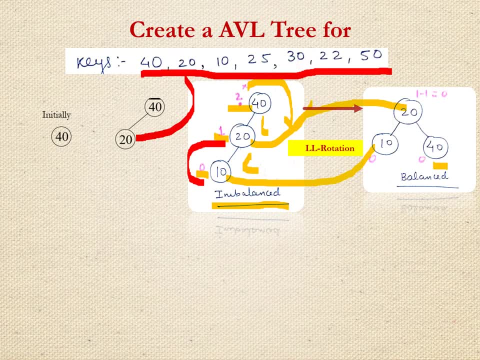 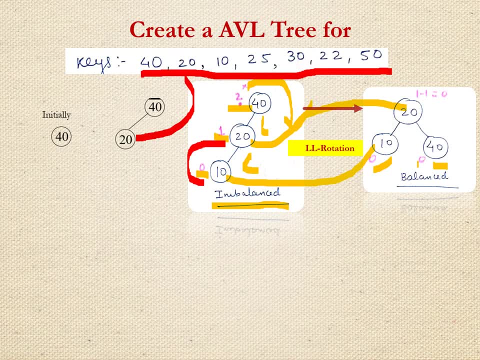 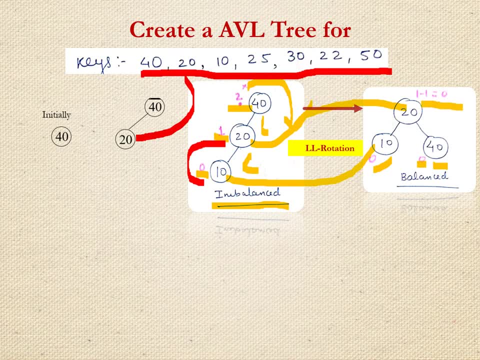 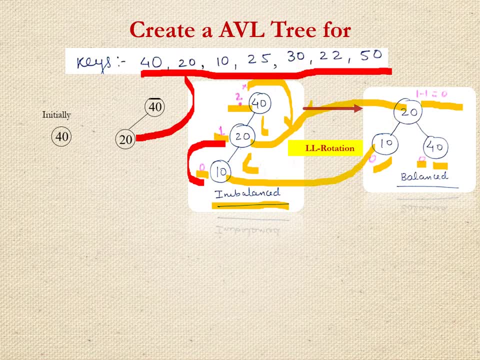 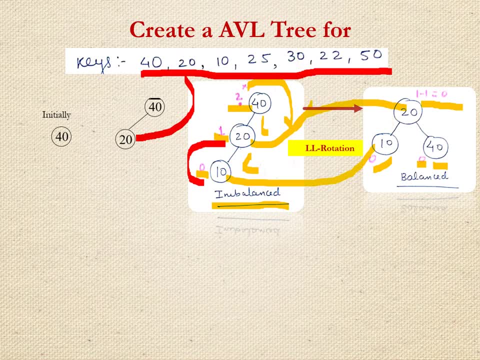 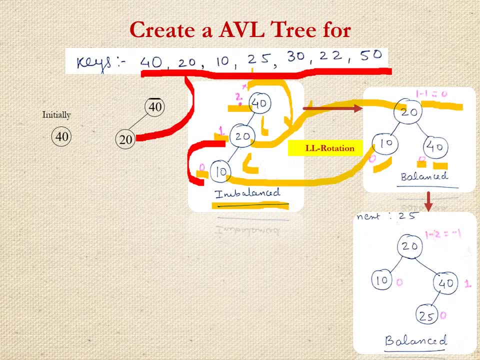 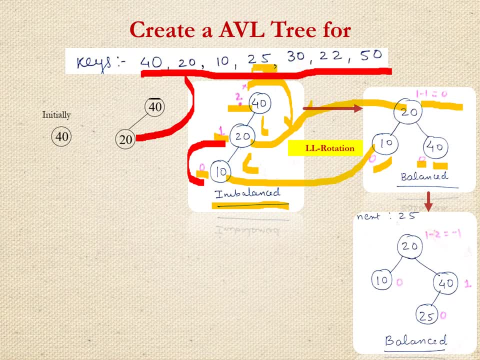 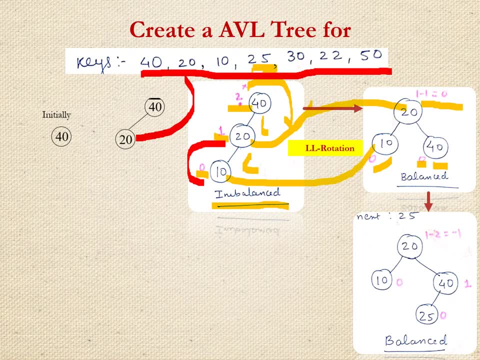 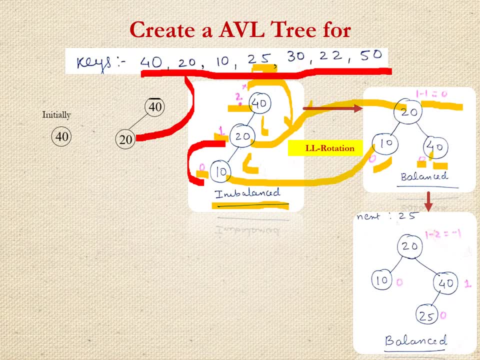 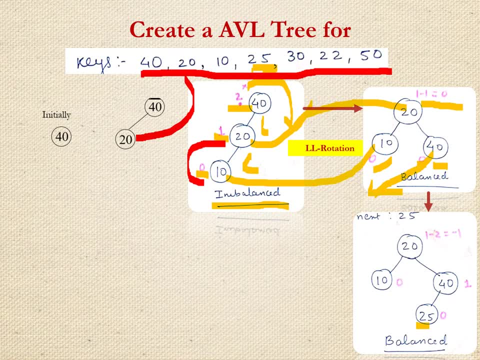 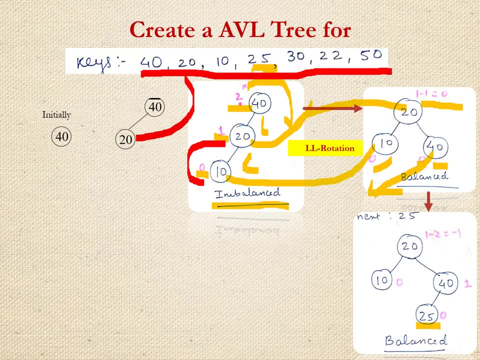 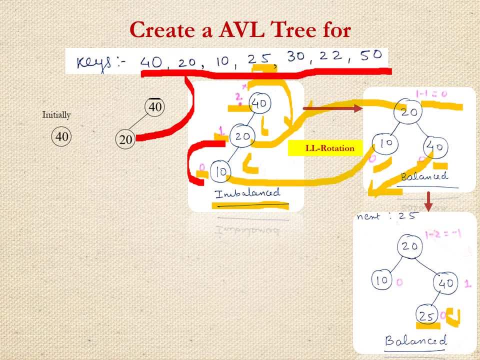 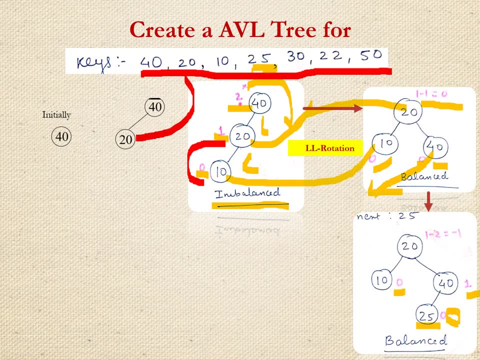 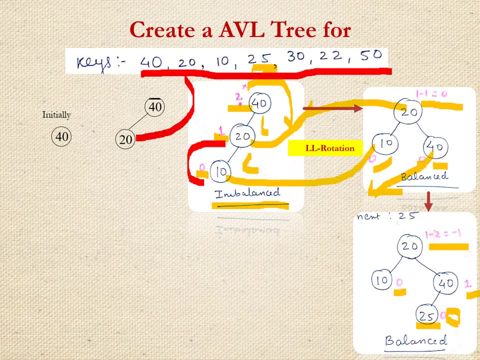 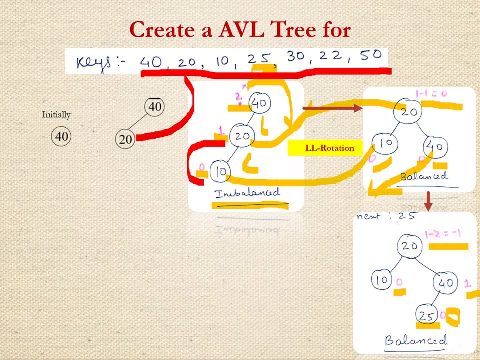 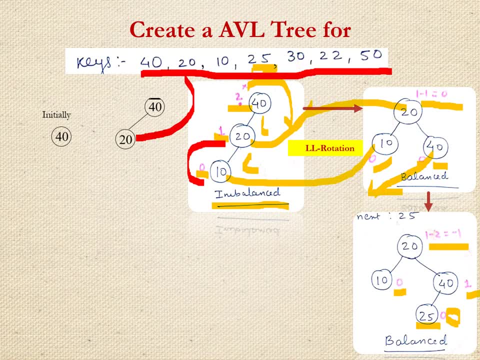 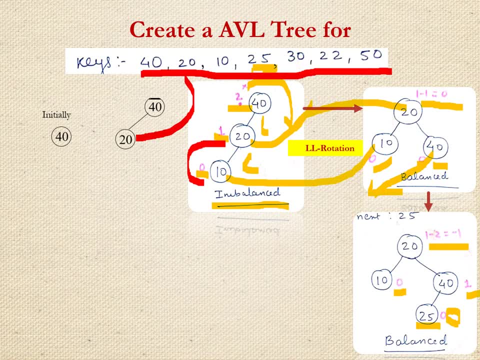 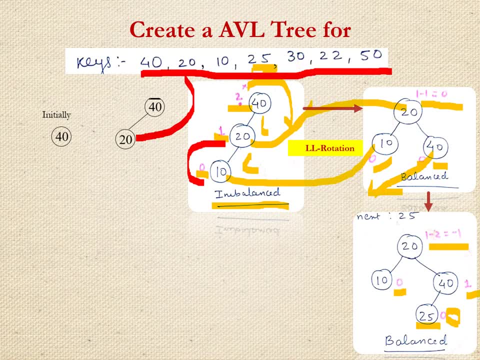 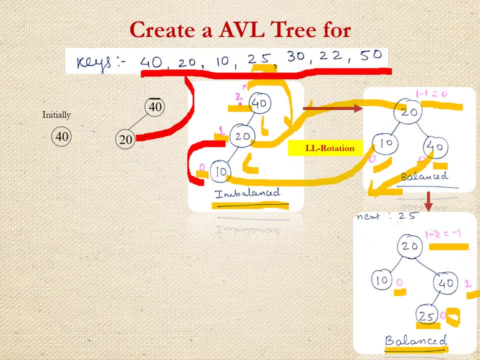 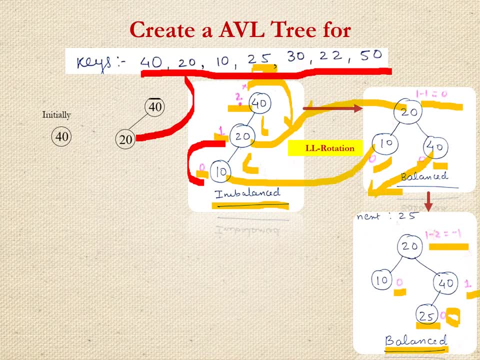 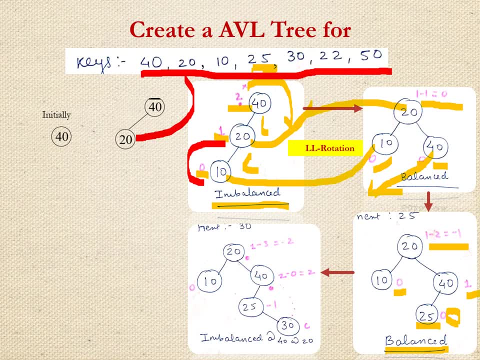 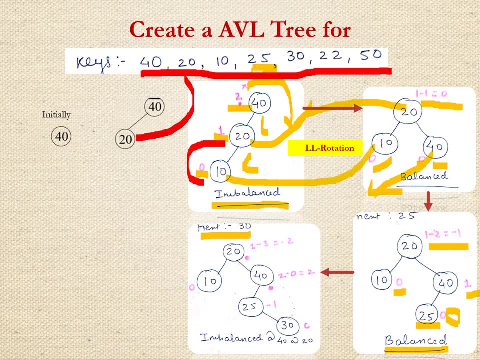 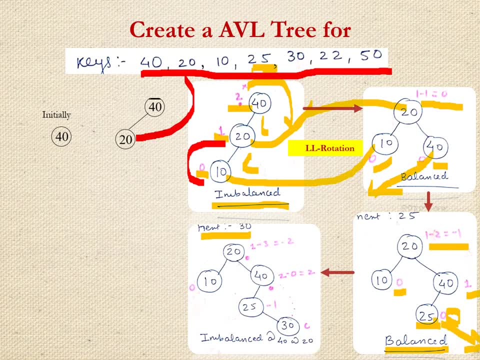 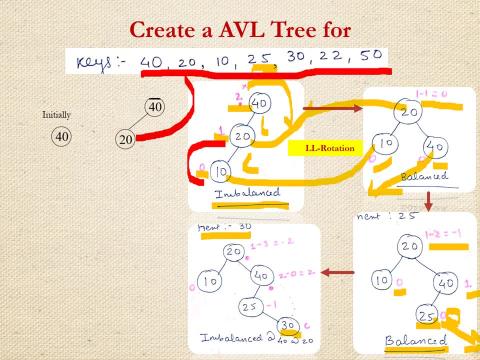 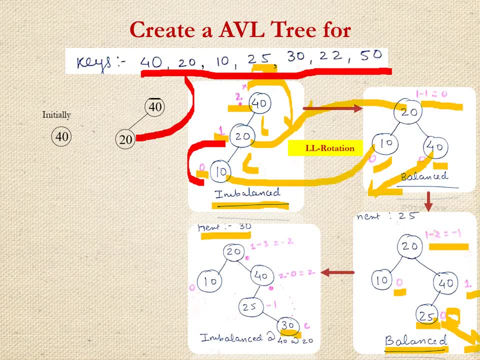 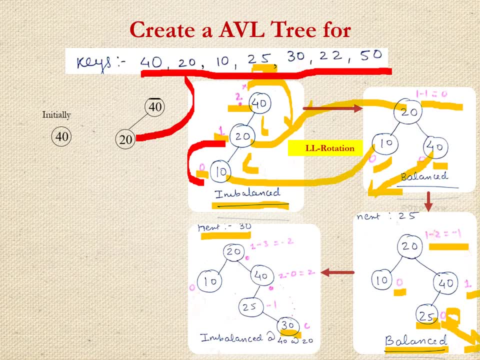 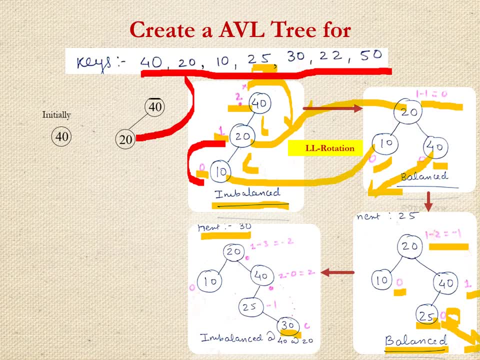 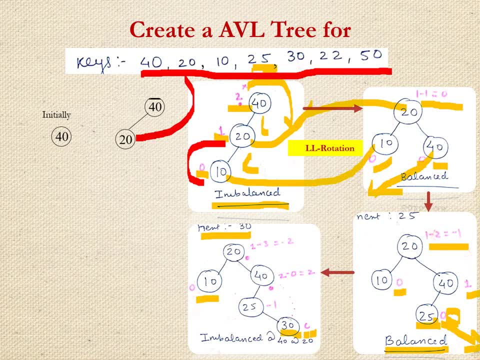 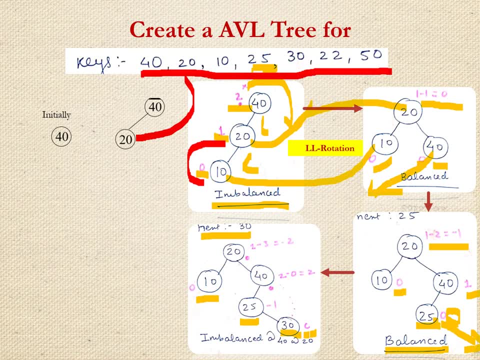 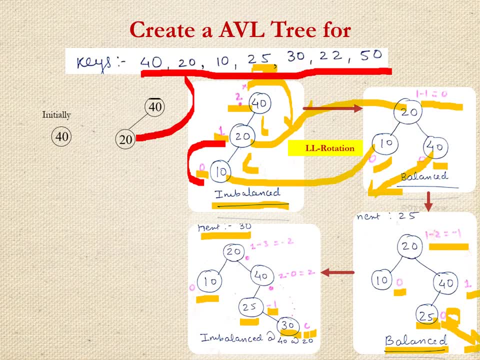 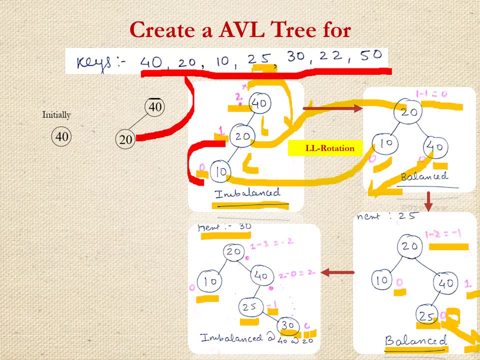 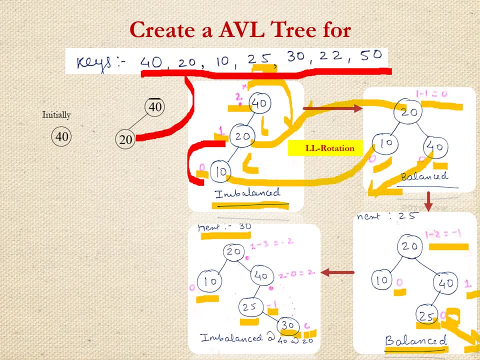 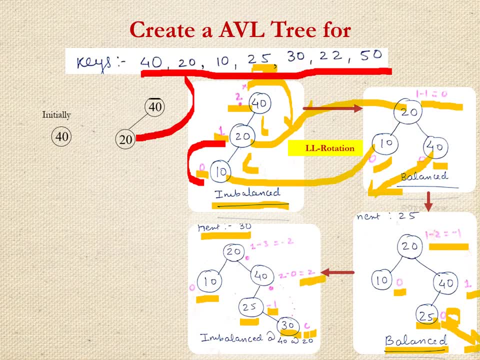 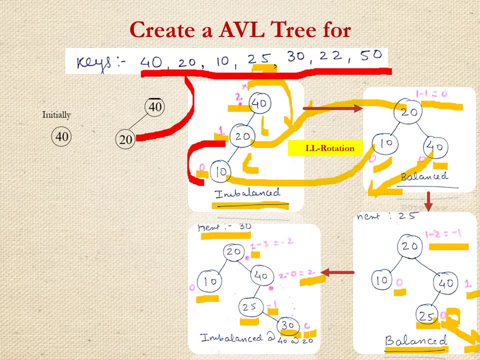 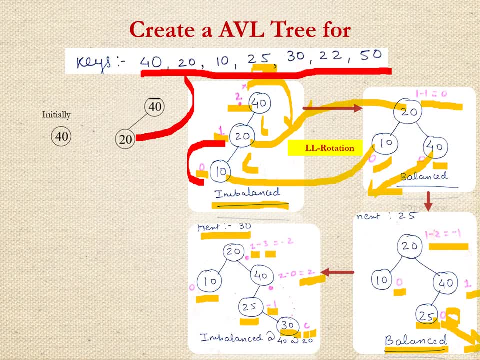 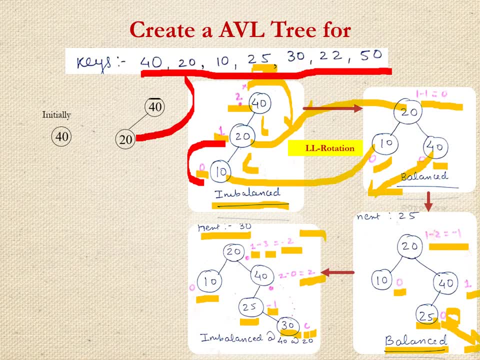 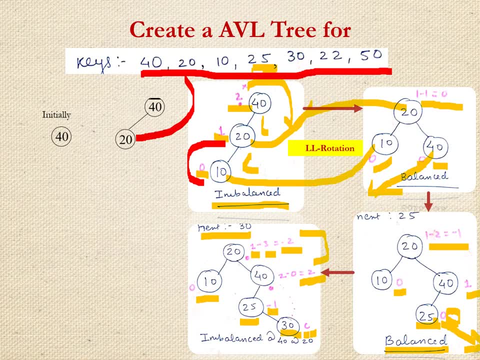 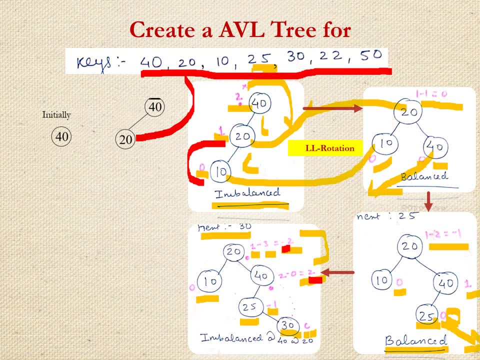 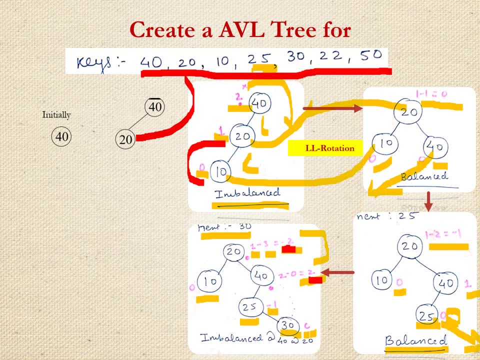 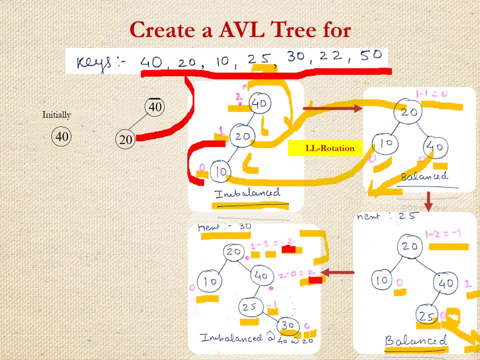 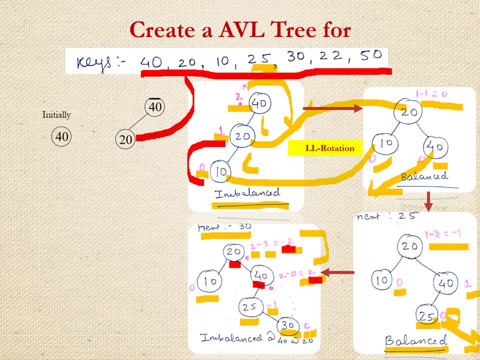 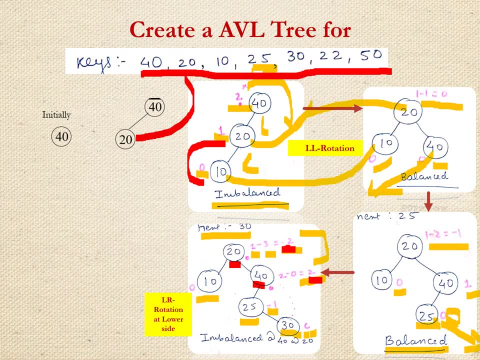 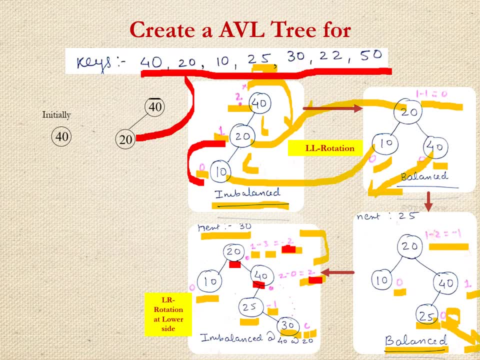 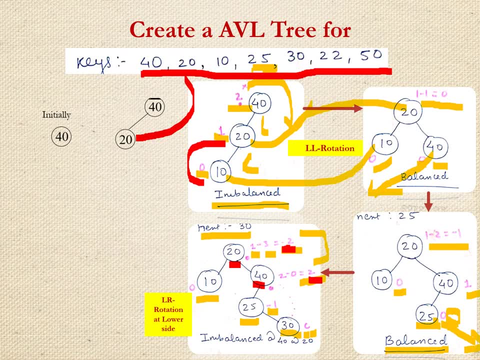 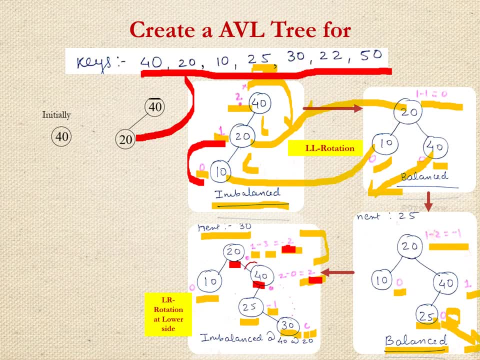 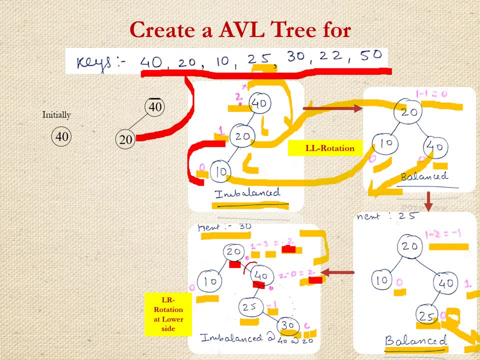 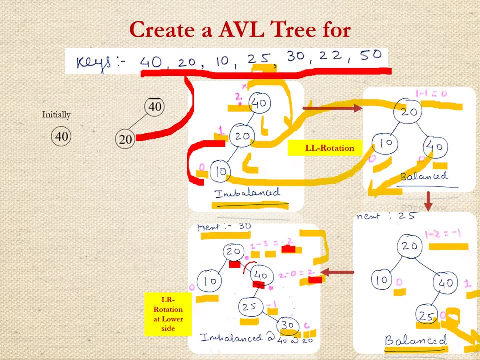 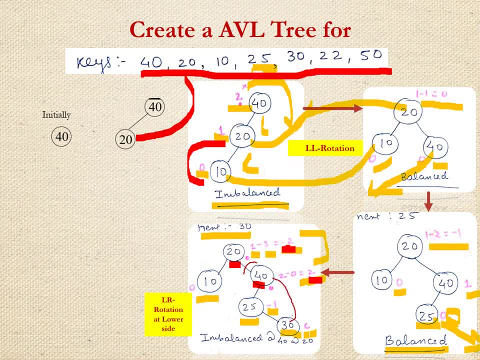 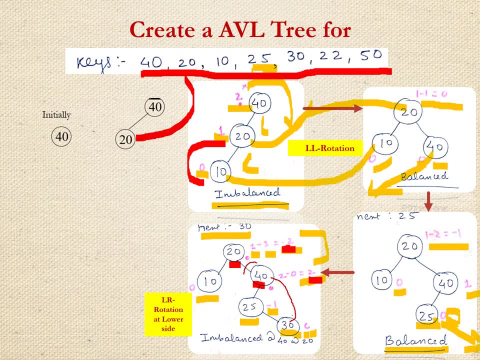 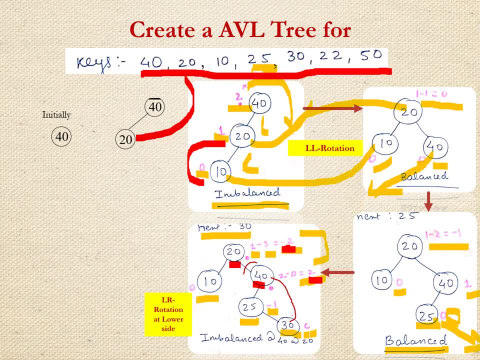 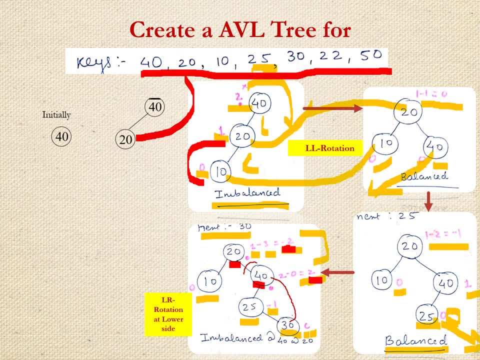 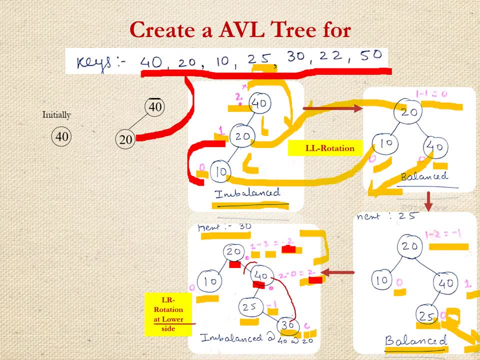 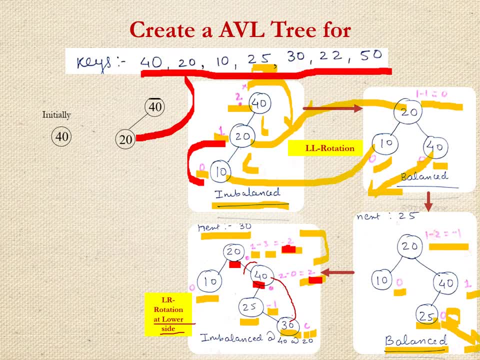 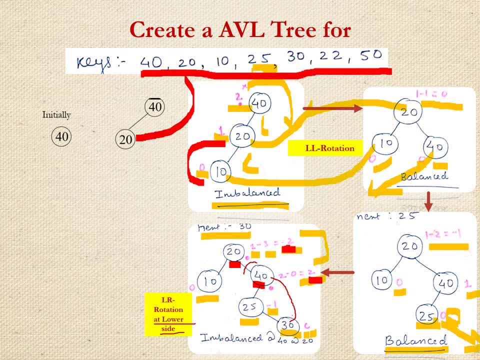 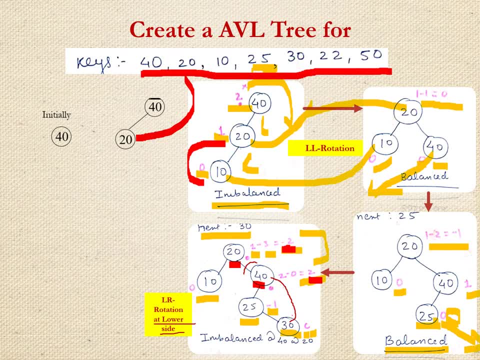 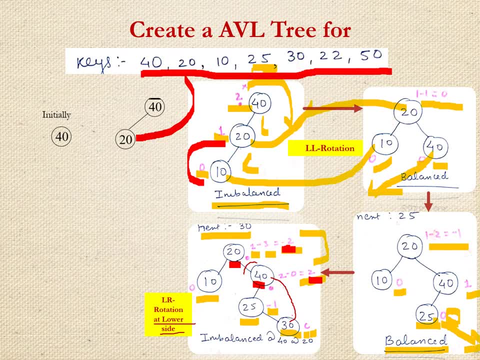 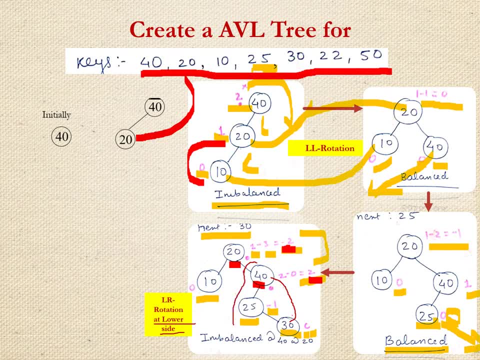 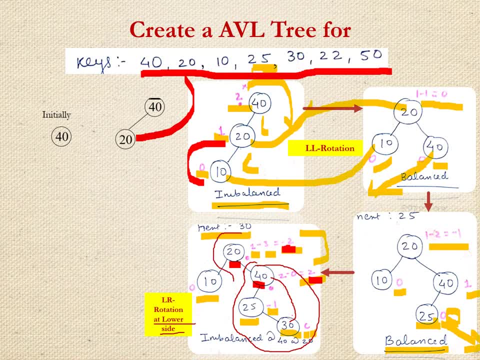 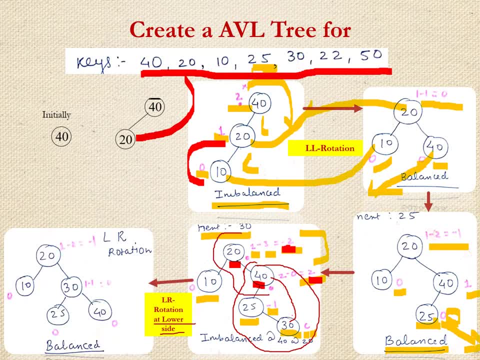 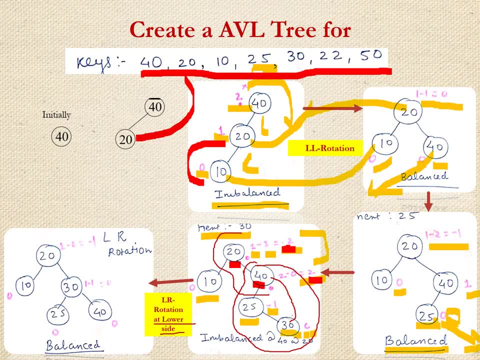 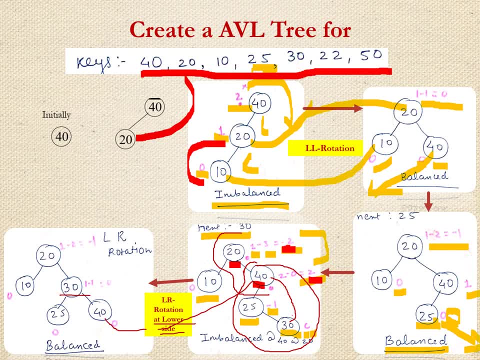 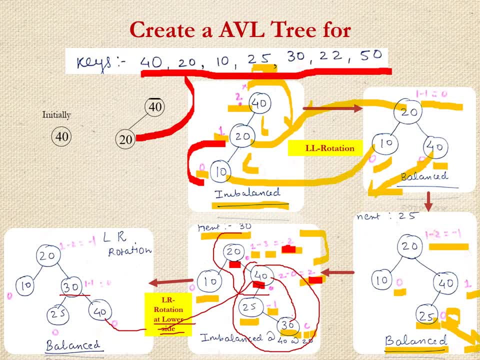 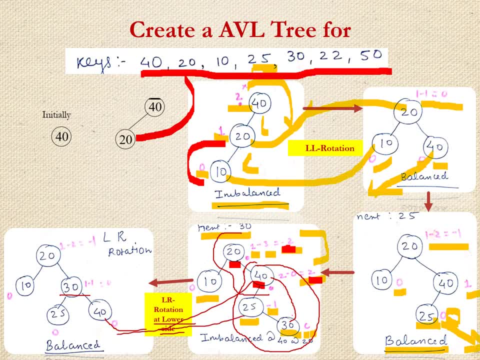 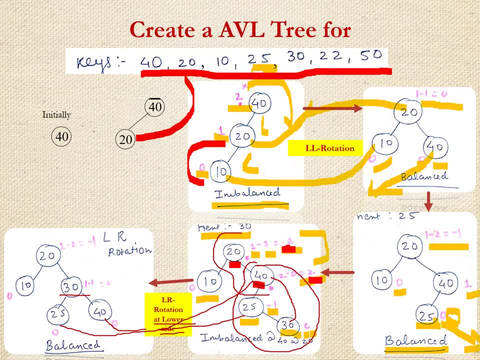 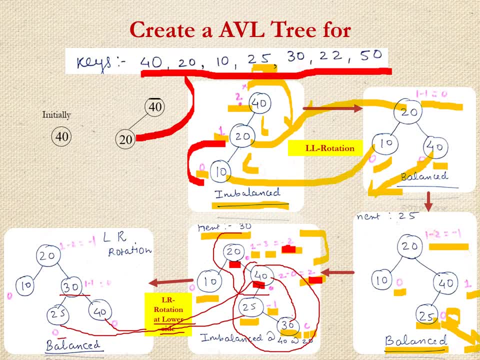 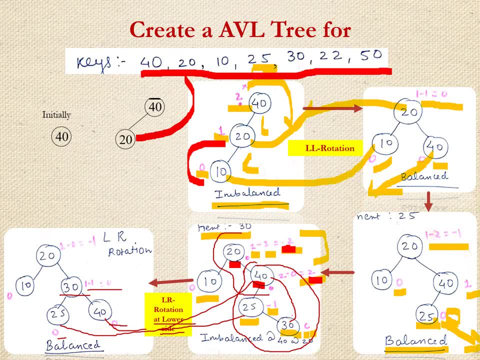 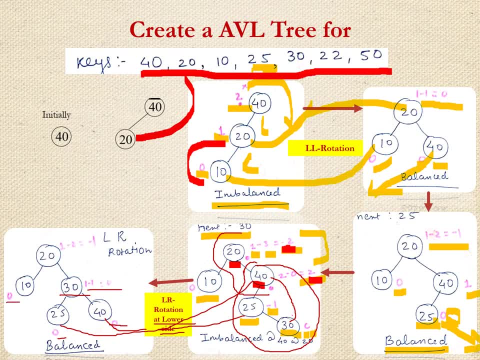 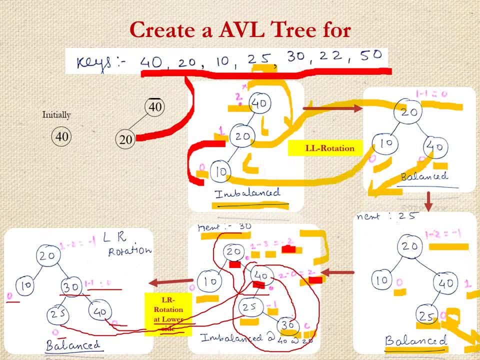 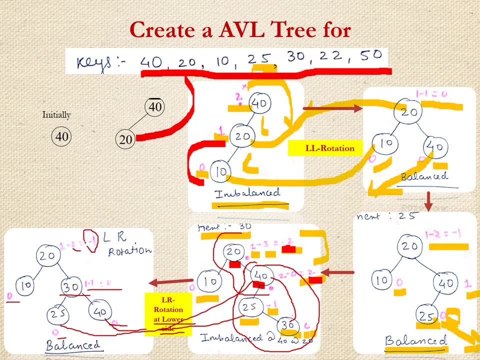 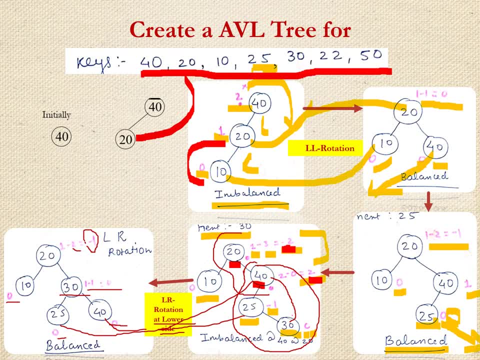 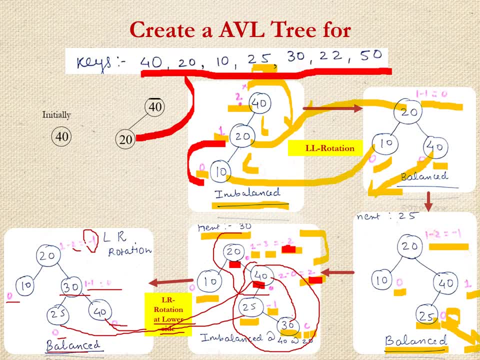 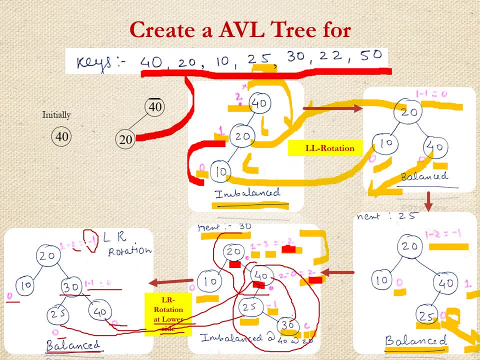 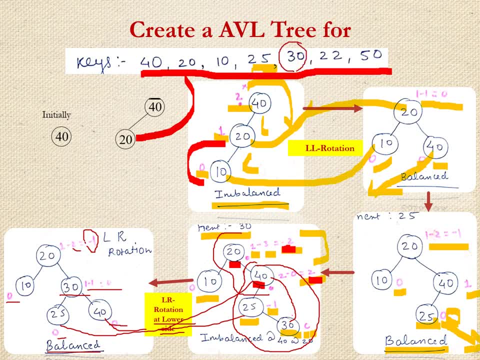 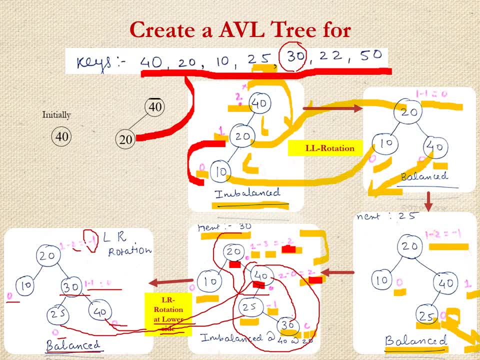 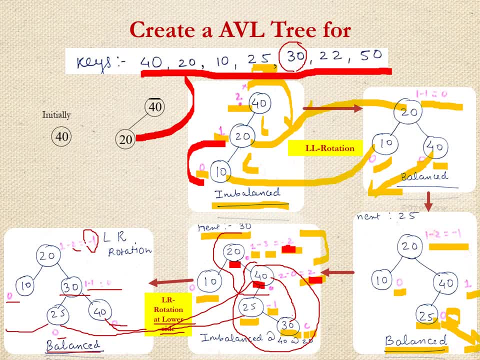 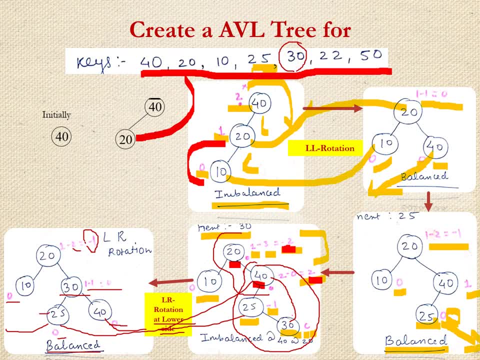 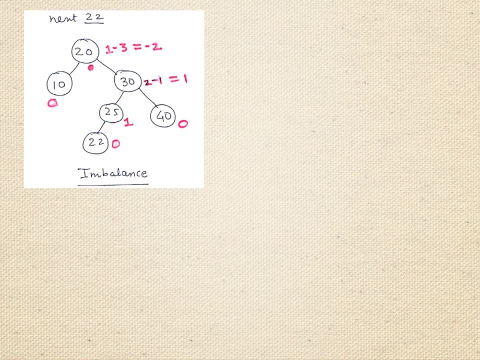 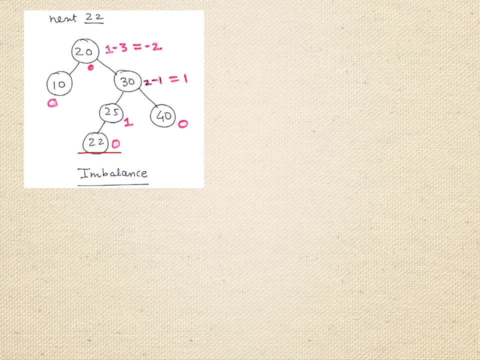 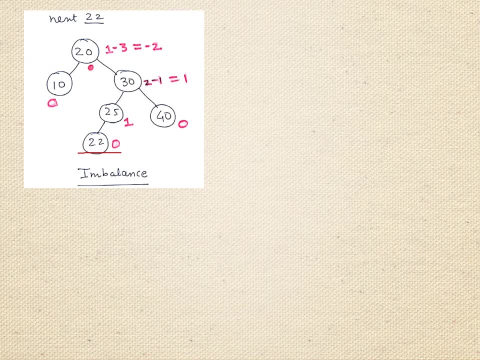 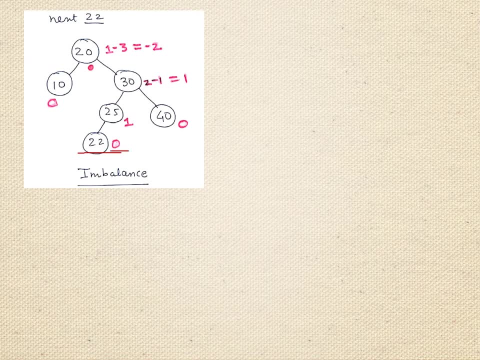 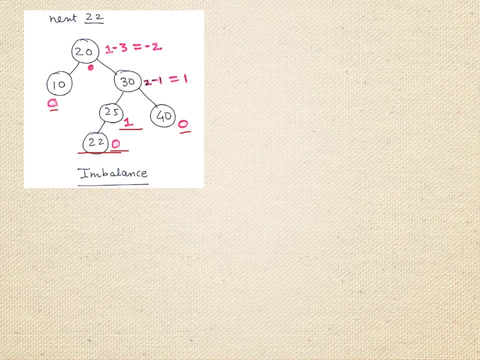 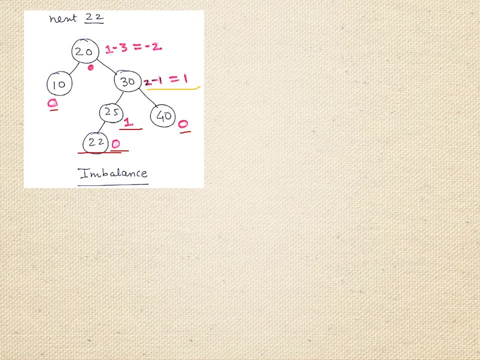 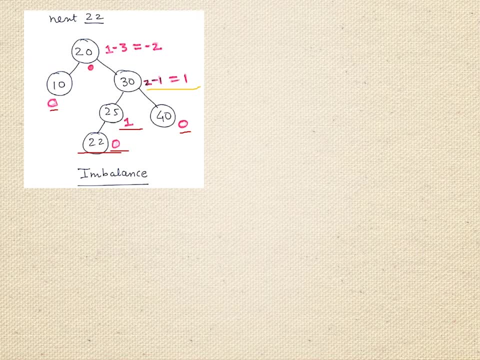 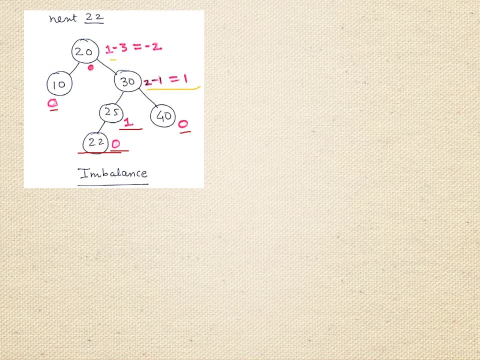 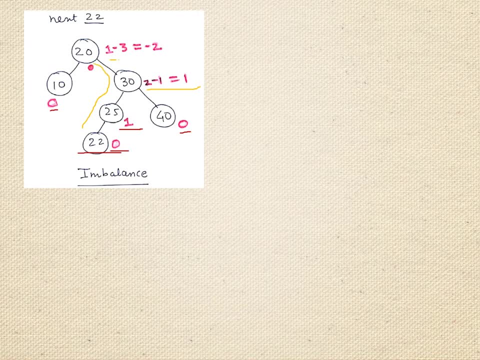 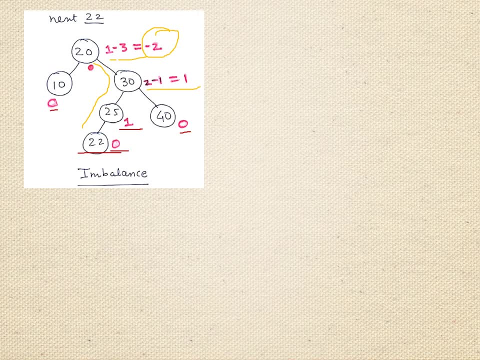 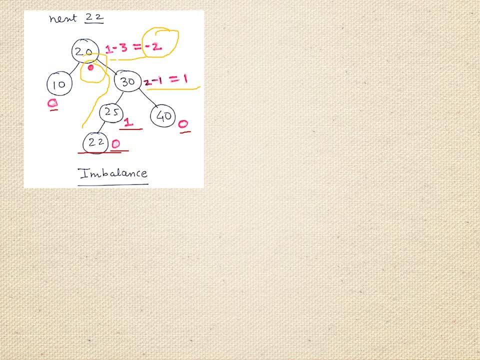 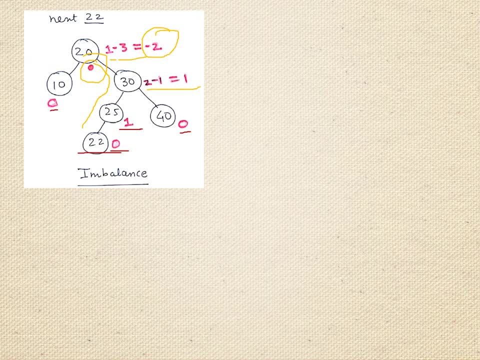 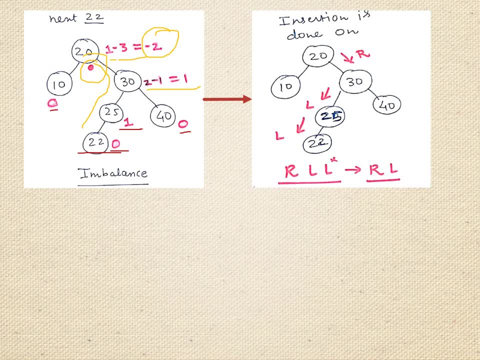 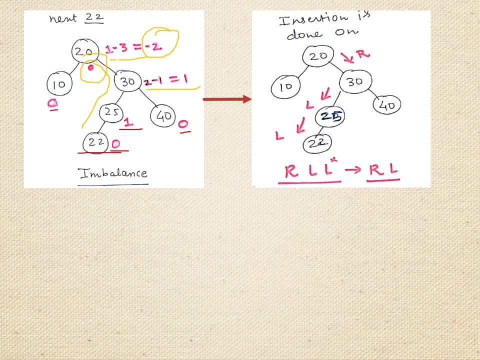 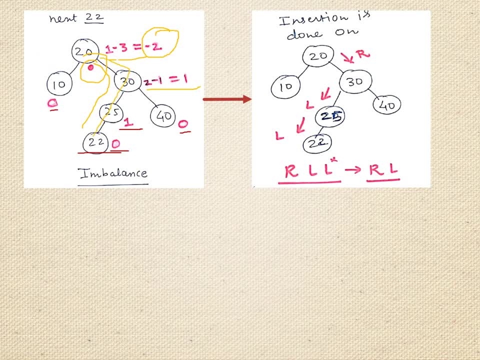 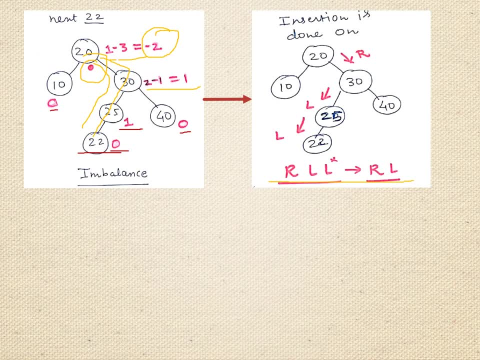 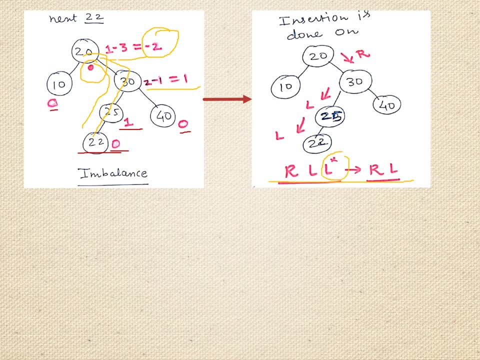 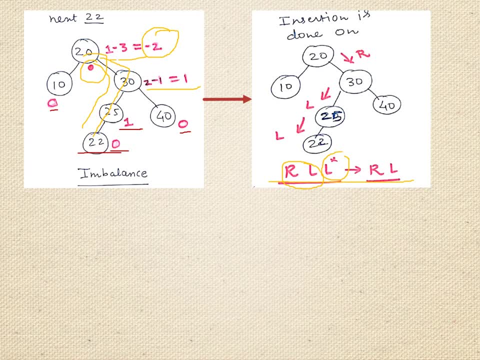 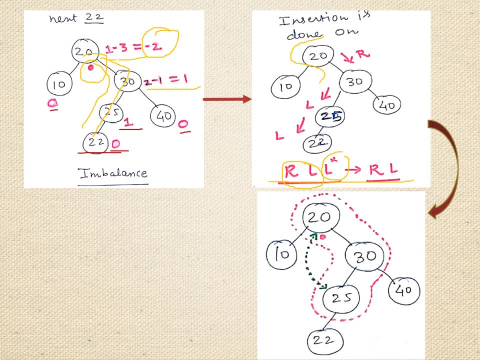 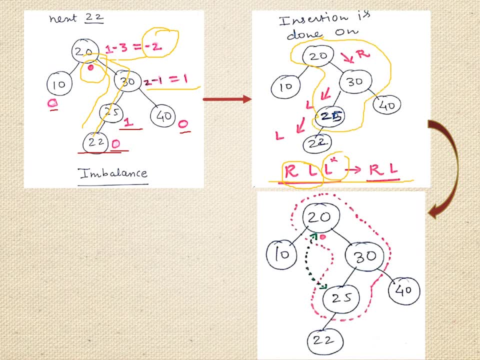 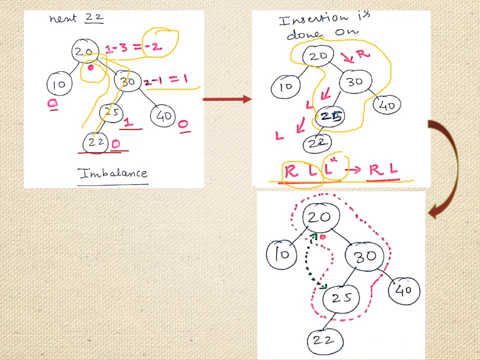 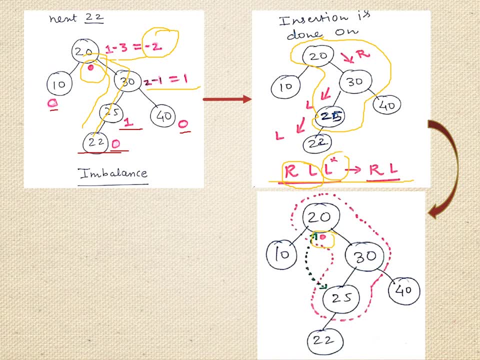 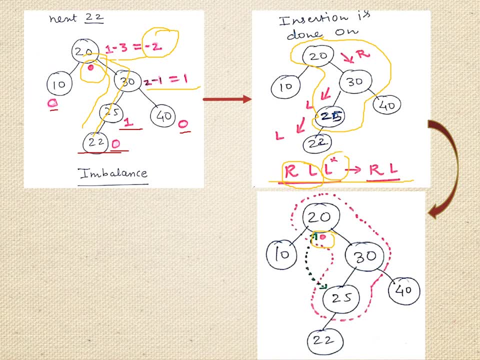 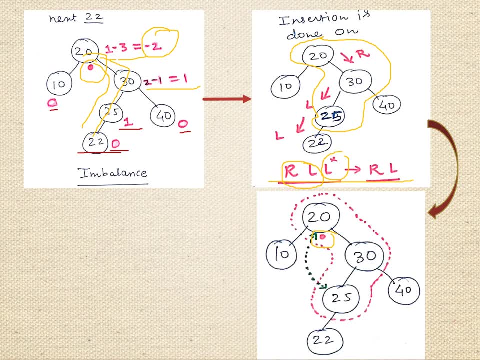 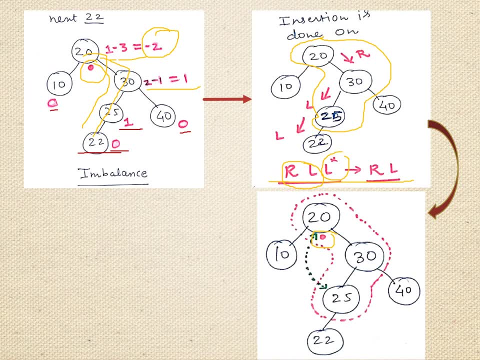 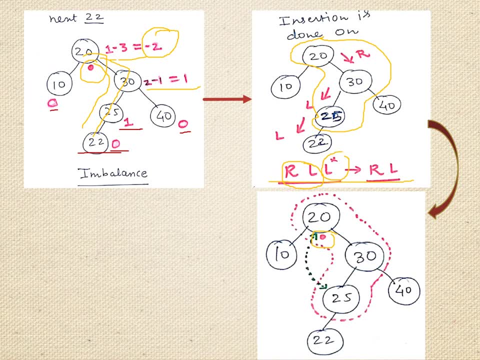 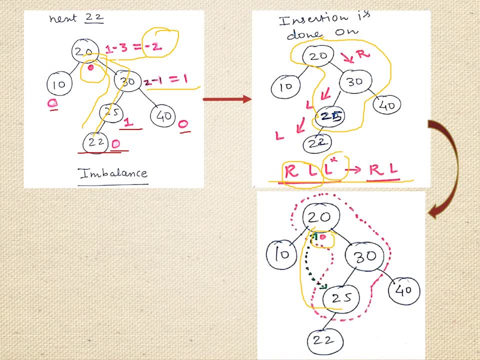 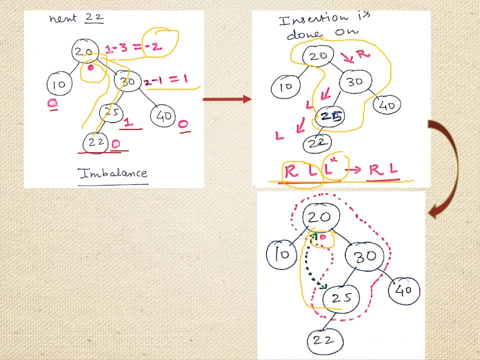 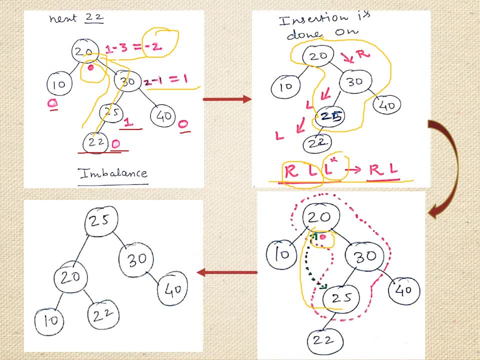 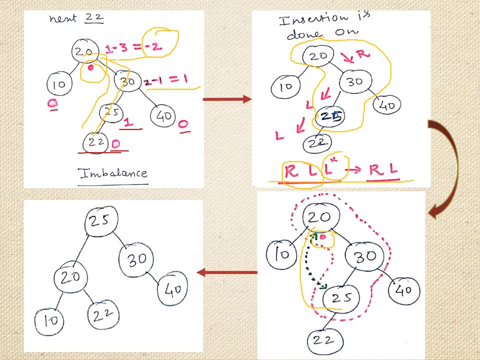 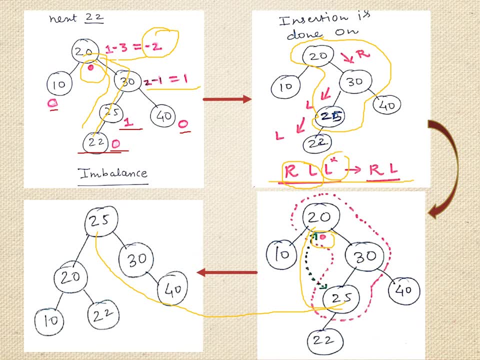 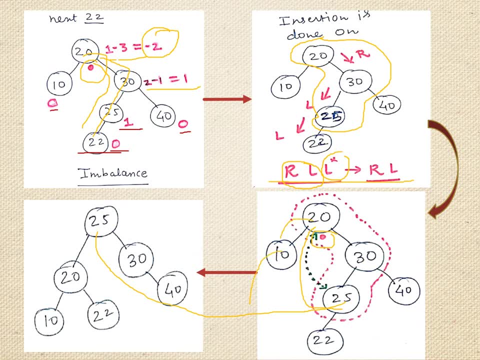 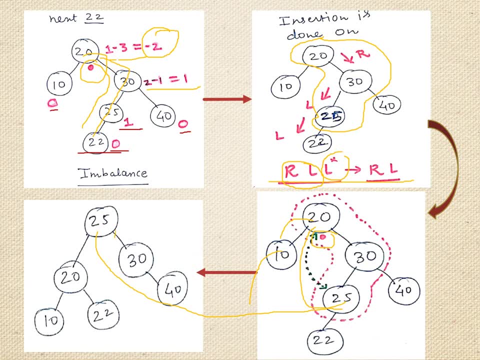 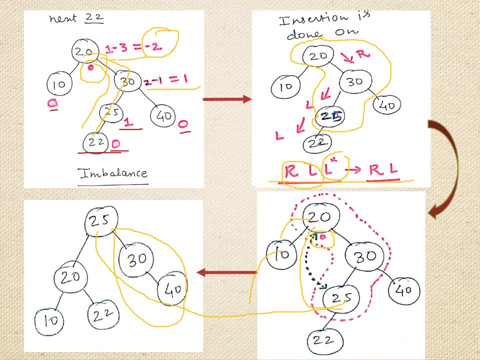 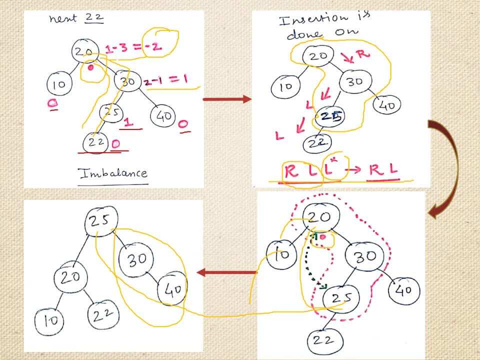 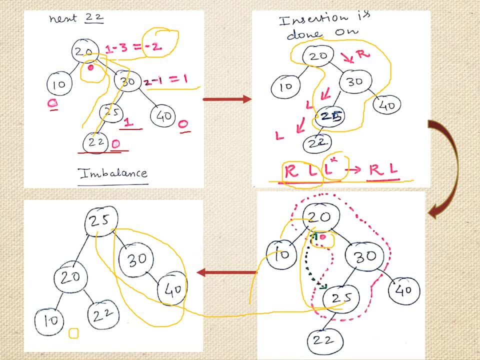 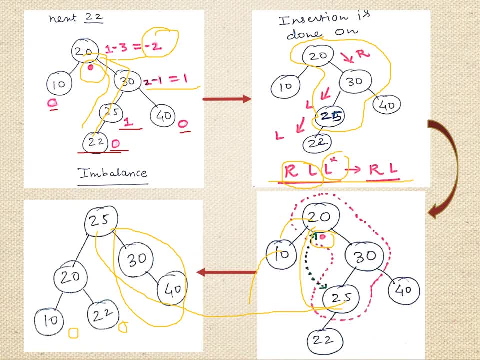 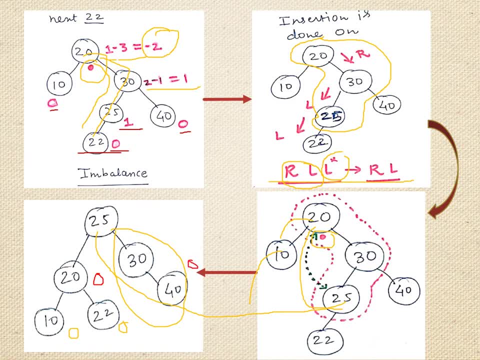 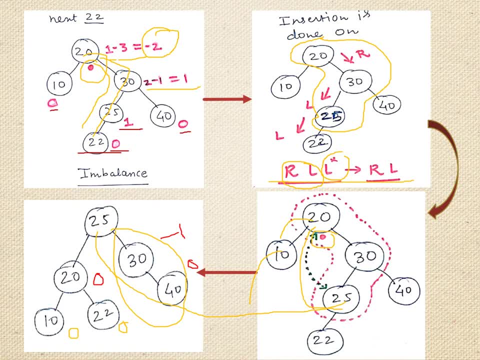 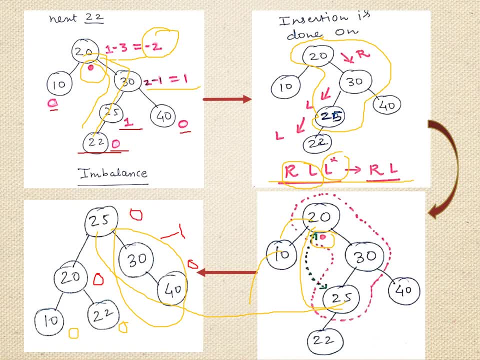 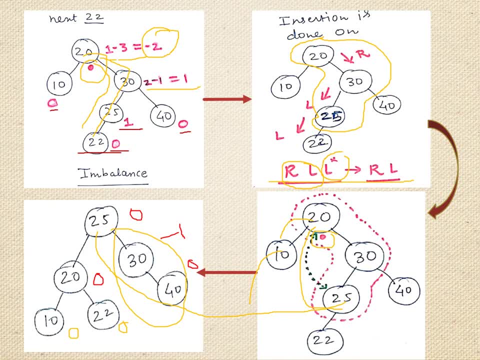 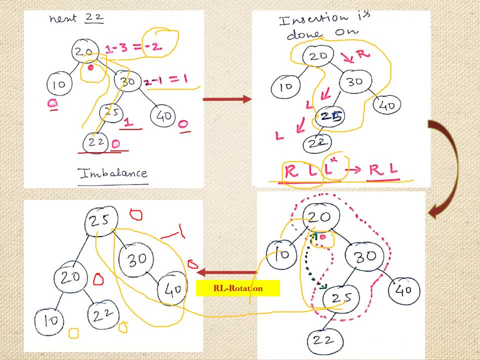 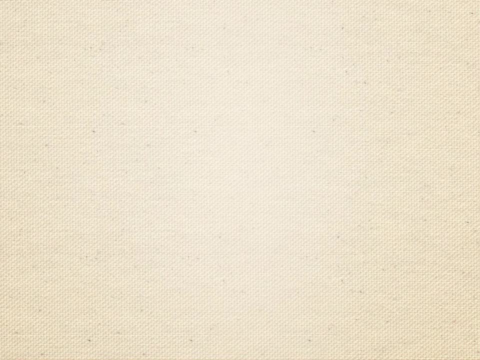 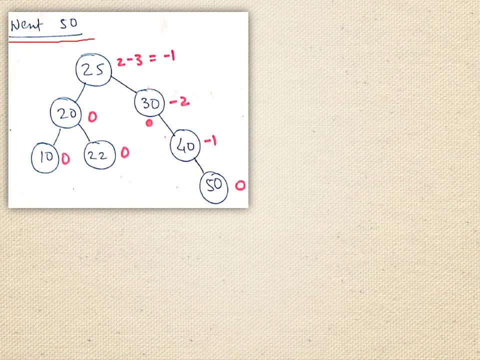 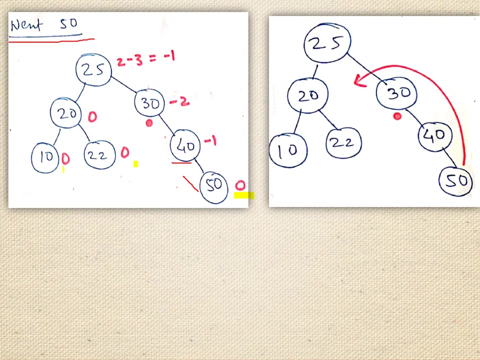 Now the next number is to add 50 to it. so 50 is the right. we can add it at the right. most of your 40. so it has added here again, we have verified all the balance factor. so verified the balance factor here. so it is something. this is 0. this is 0 for this leaf node. this is 0 for the leaf node. 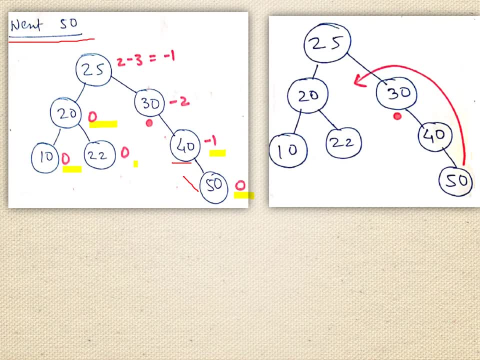 this is also 0. this is 0. this is minus 1. this is 0 minus 2 minus 2. this is 2. that is height of left subtree and the right subtree is 3. so 2 minus 3, it is minus 1. now imbalance is happened here at 30. 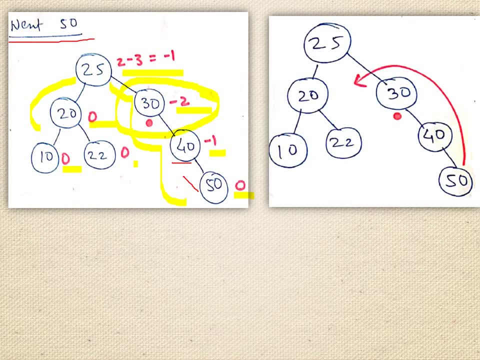 okay, that means we have to shift this 30 towards the left side so that this whole part getting balanced. so how we can do it, so you can verify, this is what, by it is done, because this 50 node is added to the right of 40 and then 40 is right of 30. which kind of imbalance it is. so it is the rr imbalance. so 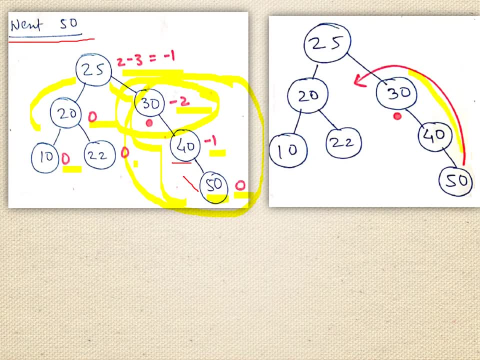 what we will be doing. we will be shifting this 30 towards the left. this is rr rotation. so what will be getting out of it? your 30 node will be shifted down, 40 will take the position of your 30 and 50 node will be as it is. 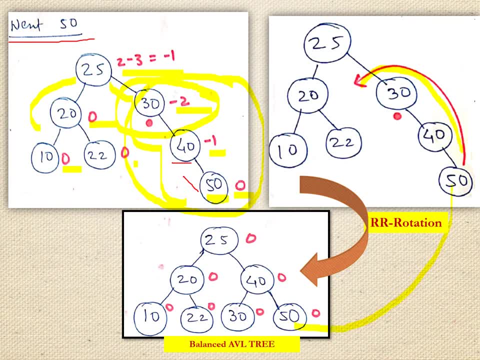 so you can verify that 50 is there as it is. this 40 is shifted upwards on the same one and then 30 is shifted down. so now 30 shifted here and then you can verify. all balance factors are 0, 0, 0, 0. 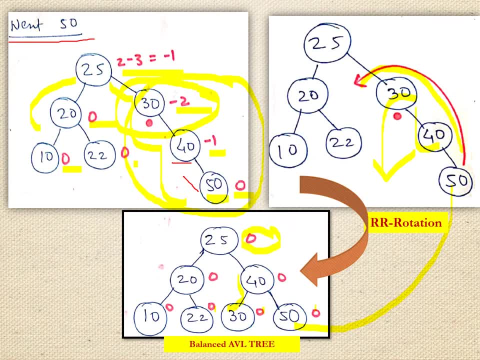 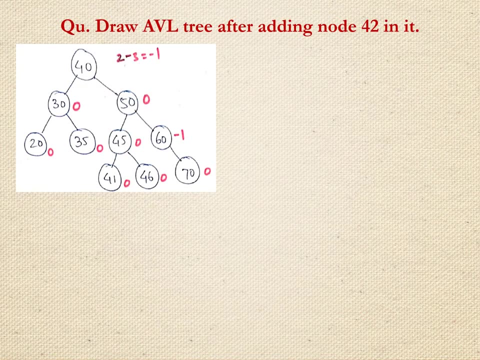 and even for the root it is 2 minus 2: 0, so this way we have got the balanced avial tree as a answer. after inserting so many nodes in this avial tree, Let us solve one more problem on avial tree. Suppose this tree was given to us. 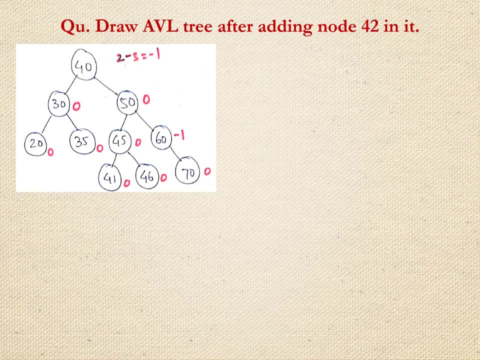 and it is asked to add a node 42 in it. So now we can compare 42 here with the root first. So that is 42 is greater than 40. So it will go right. Then it will go 50 of left of 50. 42 is less than. 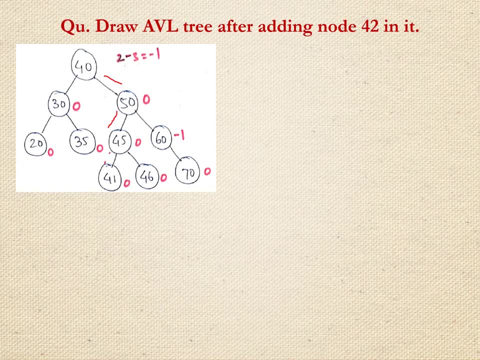 50. Then again, 42 is less than 45 and then 42 is greater than 41. So it will be added on the right hand side. Before adding this, we have to verify the different balance factors also. So we have verified here different balance factors. So it is already checked out. It is zero for the. 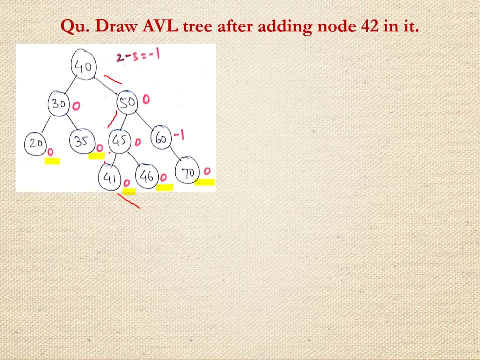 leaf. So it is already checked out. So it is already checked out. So it is already checked out. And then here it is 1 minus 1: 0.. It is 0 minus 1 minus 1.. Then it is 1 minus 1: 0.. Here it is 2 minus. 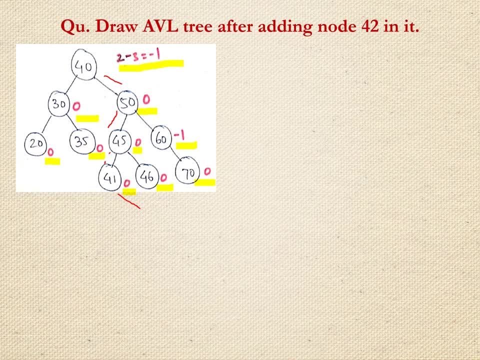 2: 0, and here it is 2 minus 3 minus 1.. Previously this whole tree was balanced, Now only we are adding node 42 here. So now this will be added on the right side of your node 41.. Now let us check. 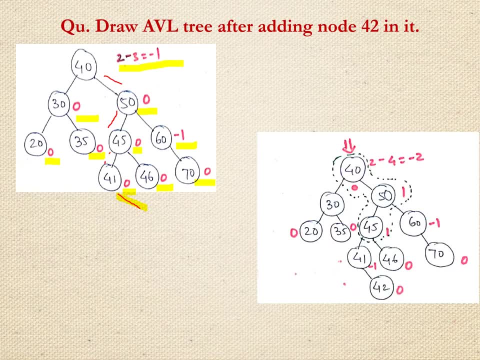 what will happen after adding the node 42 in it. So now here the node 42 is added. We have added a node 42 here, So now we can verify the different balance factor for every node. So here it is 0 for. 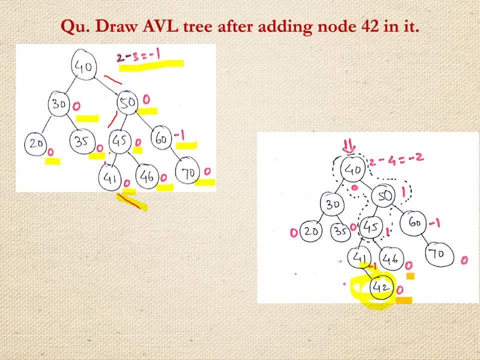 the leaf node. Again it is 0.. Here it is also 0.. Here it is 0.. Here it is 0.. Now, here it is. we can verify: 2 minus 1.. It is 1.. Here it is 0 minus 1 minus 1.. Here for this node it will be. 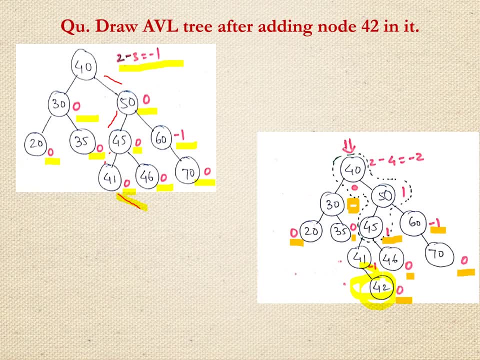 again 0.. We can write here 0.. Now for this node, here it is will be the left. height of this sub tree will be 3. And here it is 0. So here it is 0.. Now for this node, here it is will be the left. 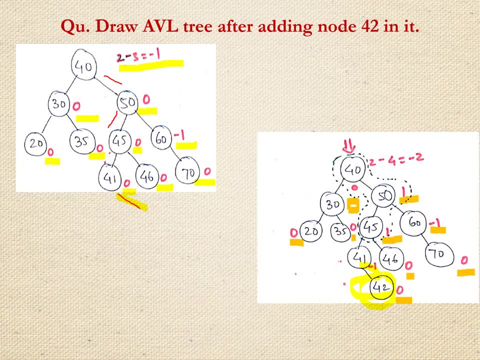 height of this sub tree And here on the right hand side, 2.. So it is 3 minus 2, 1.. And for this node it will be, left sub tree height is 2. And for the right most sub tree, it is 4.. So now it is. 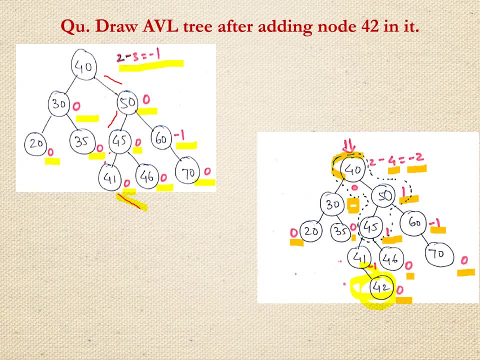 between minus 2.. That means your node is getting imbalance at the node at node 40. And this imbalance is shown here with the dot. Now what you can do, Why this has happened? Because you have added a node 42 at the end. here Means right of 41, that 41 is left of 45.. 45 is the. 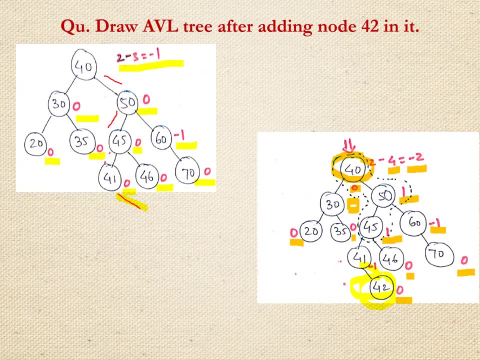 left of 50 and 50 is right of your 40. So that means there is an imbalance at the node 40 and this is the right moment here, right and again it is the left moment. So we can verify that the we have to perform the rotation or the performing the balancing in this region of the. 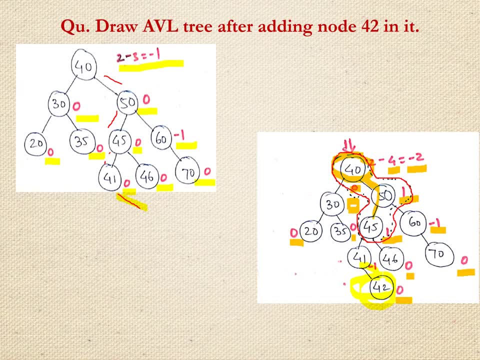 A wheel tree. Fine, So now this is a right and then a left from here, and then we are going to the left, So we are left as of a rotation. so what will happen? 45 will be shifted to 40. 40 will be there on the left of 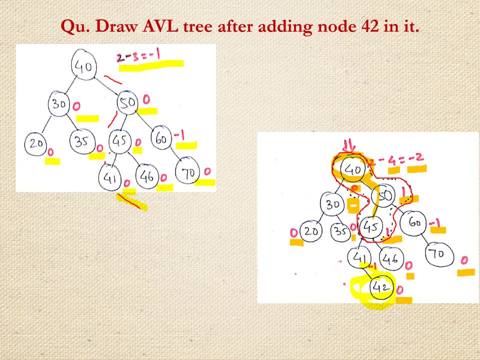 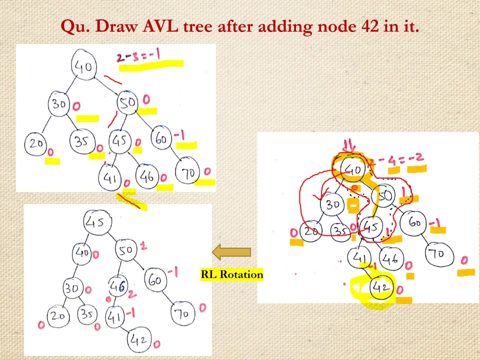 this root node and then 50 will be there as it is. so we can do it, the shortcut, we know it. so this will be: 45 will be shifted here, and then this 40 will be here before 30 and then the rest of arrangement will be the same. so you can verify, we did the rl rotation so we identified 45 is. 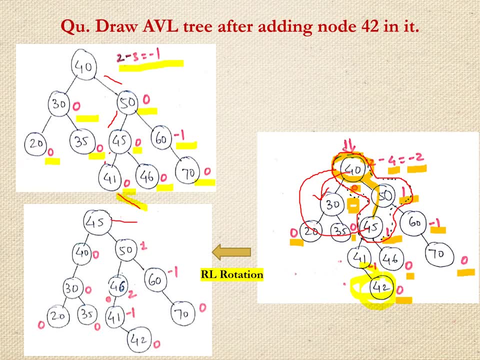 there now on the top, that is, it will become your current root, then 40 shifted to the left hand side, then 50 is on the right as it is. so this is a rl rotation. in short, we did it and the rest for rest, balance it factor we have identified. so, again, after identification of the different balance, 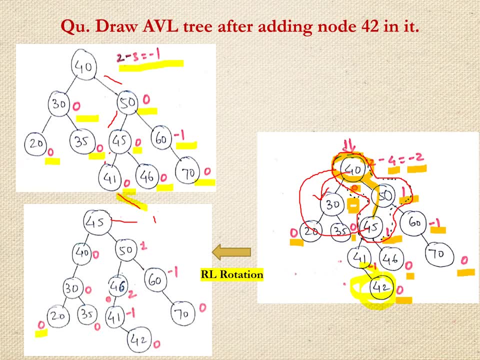 the factors so we have identified. for the, the leaf node, it is 0, it is 0 0 0. now this is 0 minus 1 minus 1. then here it is, with the what we can: 0 minus 1, it is minus 1. then here it is. for the left of, it is 3, 2 minus 0, it is 2. 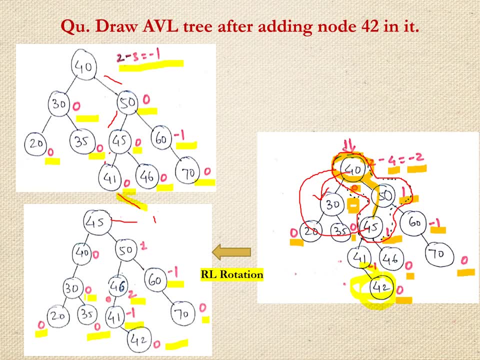 then it is 0, 1 minus 1, 0, here it is 0, here it is 1, and the rest you can verify. here it is 3 minus 4, so here it is also minus 1. so but here we are getting the imbalance. so here for we are getting. 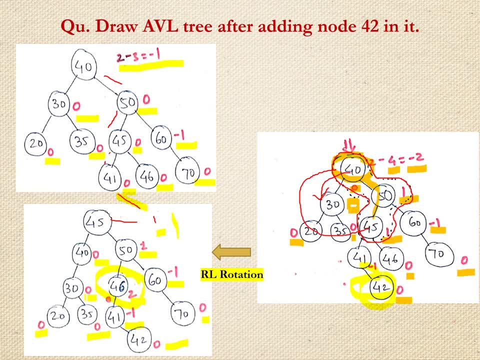 the balance factor, uh here as 2, so we have to balance it. so which kind of uh rotation we can perform? so you can verify: here it is l that is. 41 is a left of your 46, so that way we have identified it as l here. here it is l that is this one. 41 is left of 46, so it is l. and then 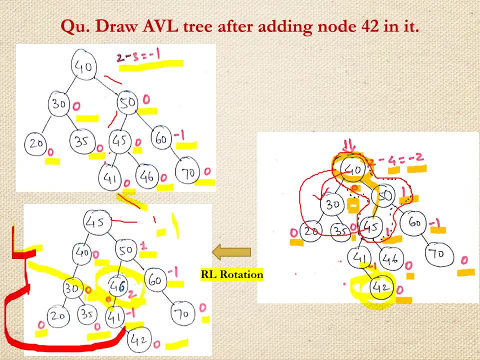 we have here the right-hand side of this. this is 6 and it is right around variant laws. now what we do is to write the difference between each of these VIF, the integration values. so let us prove again here. that is here. it is not a type, and so we have given. 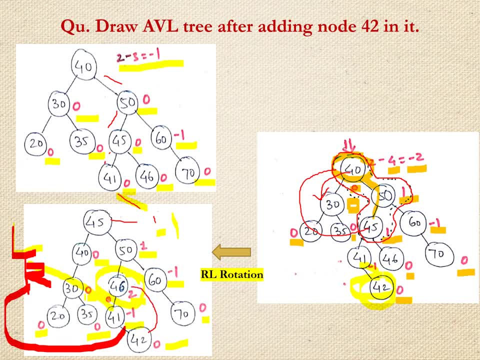 itself as a point, so that we can get a difference between which part we areikum al detail, as it is, form the current size of the property, because part of the property is right on this. well, if we can wertangerize this right of your 46 and give you a better of the from. 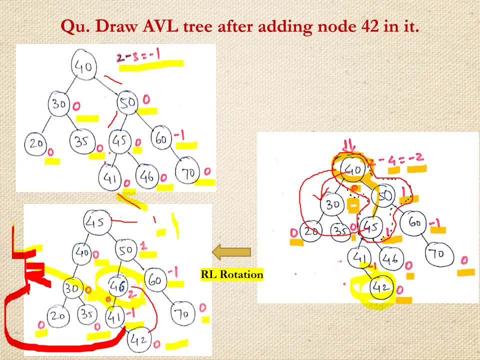 this and here the in which side it is leveling. so what we want to do, we want to take in decision and provide this equation was: what, what should be right? and asking to decide. 2ортot of the. it will be swapped first, and then 46 will come to the right of your 42. so this way we'll be getting. 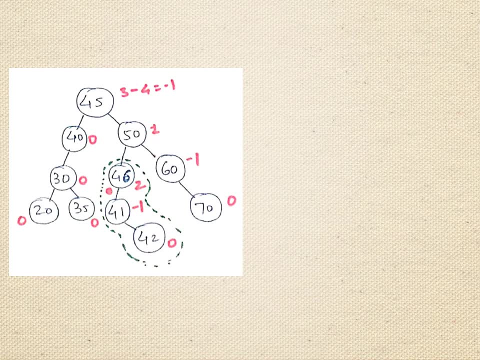 here this from the previous slide. it slipped. it is the same way, so we are shifting here on the right of it. so please verify the answer. it was imbalanced because of this two and we are performing here the l r as a rotation. that is a left, here left and here it is r rotation, so please verify. 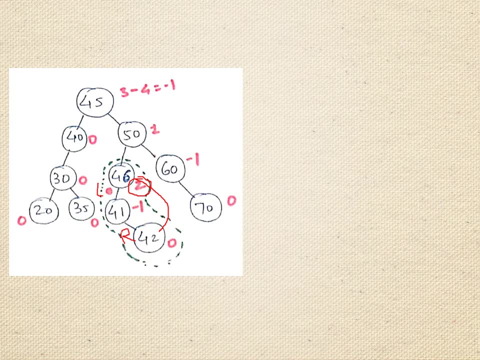 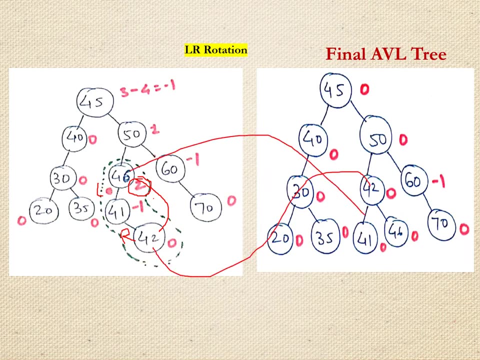 the answer. so 42 will be the root of this then, and 46 will be shifted to right. so please verify that. so we'll be getting here. there's 42 is now changed to here and your 46 is shifted here, and then 41 is as it is. so this way, we can use the shortcut that we have already seen in the in this. 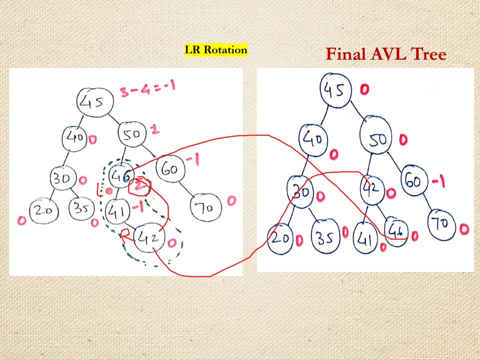 video in the initial slides and that way we can verify the answer. now again, you verify all the balancing factors. so it is all the factors are means all evolutions will come to the left and we are performing very simply. so we are Kin meno value. everywhere you are getting, it is balanced 0, 0. only here we are getting minus 1. yes, but it is in the